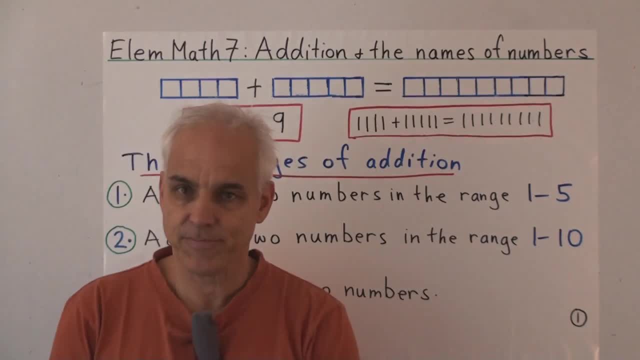 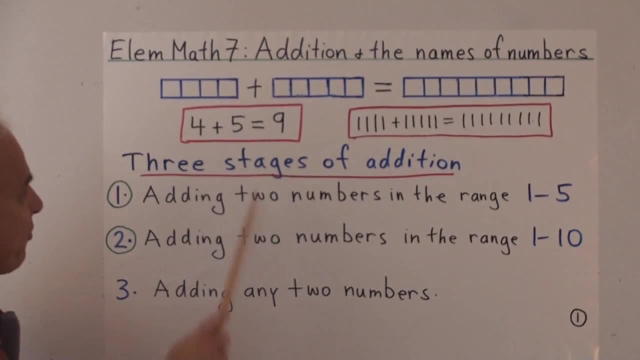 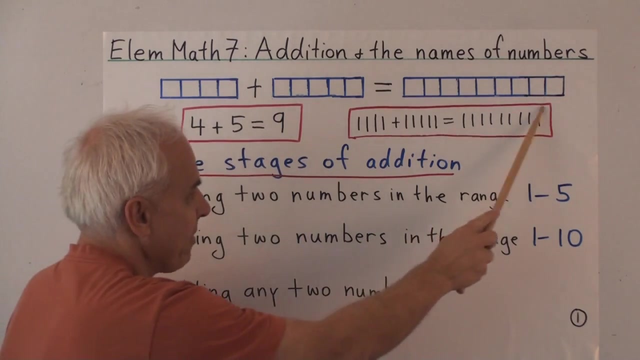 issue relating to the names of numbers once we get past the numbers up to ten. So here's a very primitive example of addition. We have this number plus this number equals this number. This is our primitive kindergarten approach to numbers, simply as rectangles. 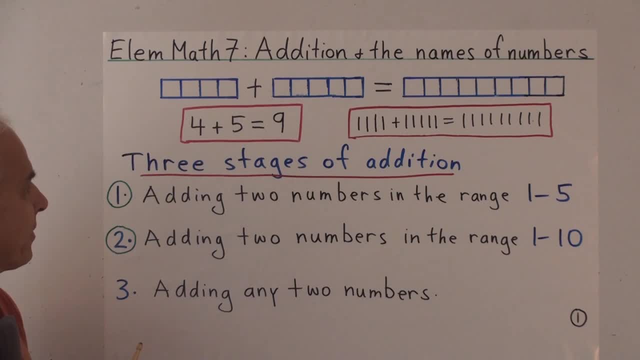 or strings of squares. And the way we add them is geometrically very simple: We just concatenate the two strings together, push the two rectangles up together so that they are one. So in the Roman system these two numbers are represented by these strings. 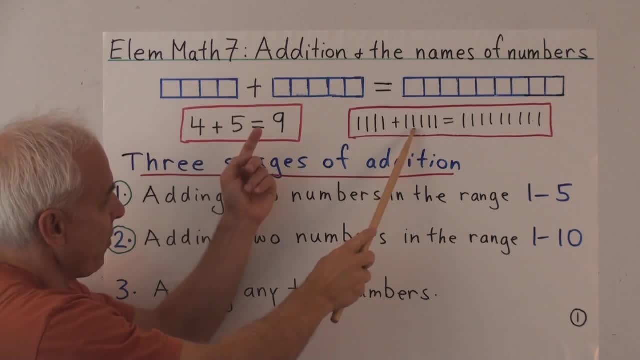 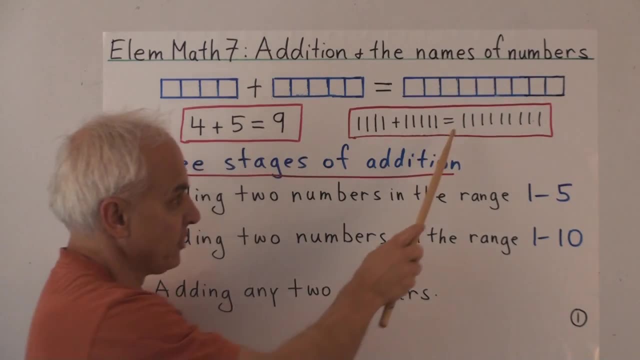 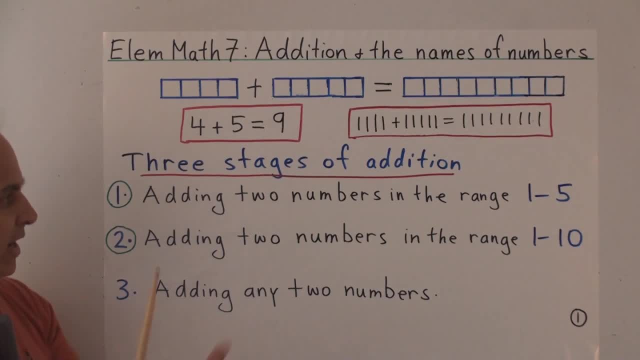 one, one, one, one. Okay, so then we ended up giving names to these numbers. So this is really the number four, This is the number five, This is the number six, This is the number nine, And here's our Hindu-Arabic symbols for those. So we would today write: 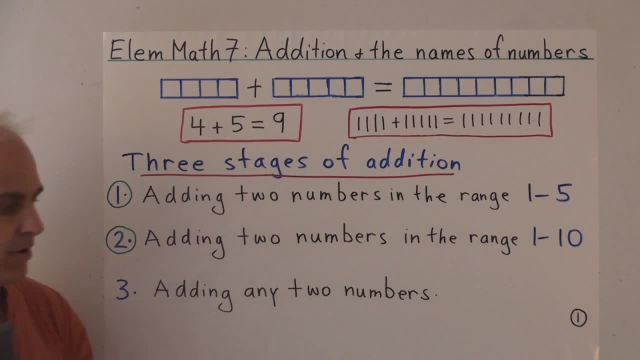 four plus five equals nine. So that's one example of the many facts that young people have to learn. They have to memorize that so that it's second nature, So that they don't even think about it. You ask them what four plus five is, immediately they say nine. Okay, 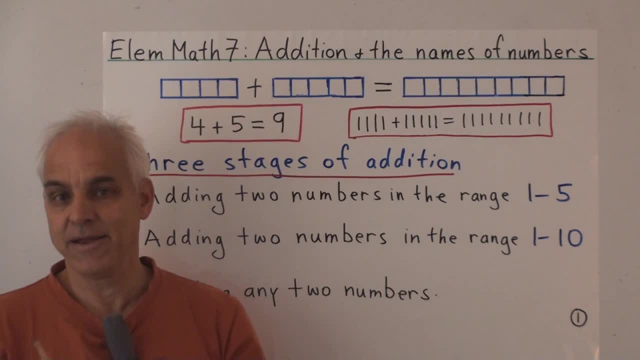 in my opinion, there are sort of three stages of learning. The first stage is the issue of adding two numbers which are in the range one to five. Like here, these numbers are both in the range one to five. This is a particularly simple. 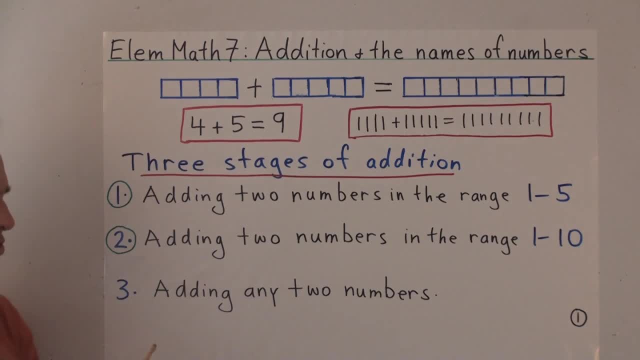 kind of addition. I think it's good for learners to start with numbers in that range And then the next step, which is really a step up, is to add two numbers. So the first step is to add two numbers in the range one to ten. It turns out that's quite considerably more. 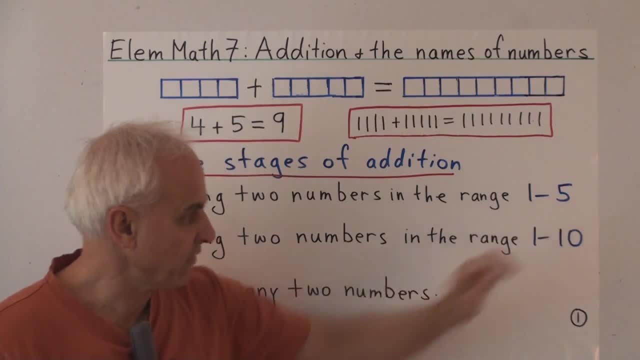 sophisticated. So students should start with addition in the range one to five and then move up to addition in the range one to ten, And then only after that. the third stage is moving towards adding any two numbers In this lecture. today we're going to be just. 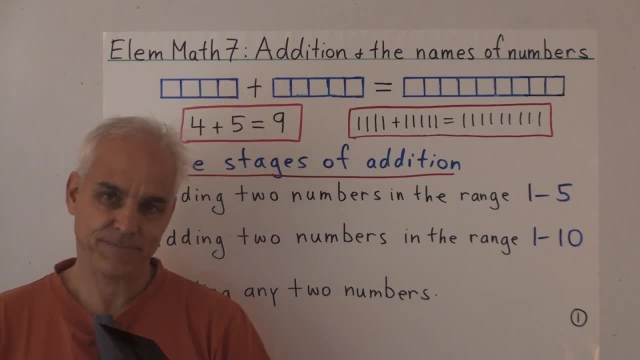 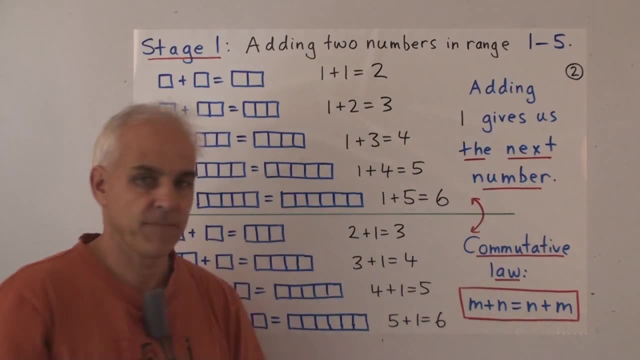 talking about these first two stages of addition. So let's start with stage one, Adding two numbers in the range one to five. So we want to do this in a systematic way, And so it makes sense to start with the case when we're 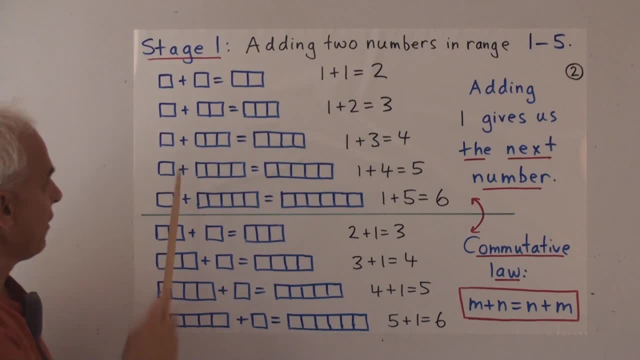 adding one to a number, For example one plus one, or one plus two, one plus three, one plus four, one plus five. It's not too hard to work out what these things are, of course. One plus one, we just bring the squares together, we get two. One plus two, bring the squares. 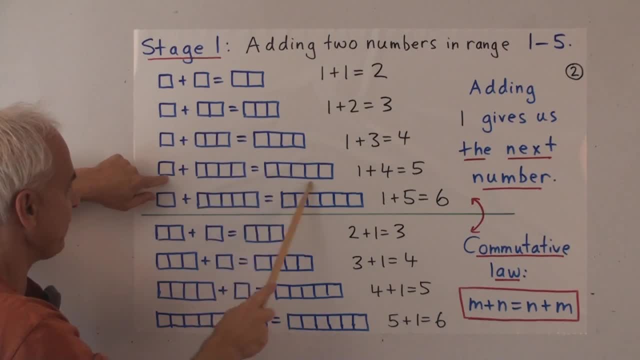 together we get three. One plus three is four, One plus four is five, One plus five is six And they are the corresponding Hindu-Arabic equation representing the same thing And, pretty obviously, adding one is very simple because it just gives us the next number. 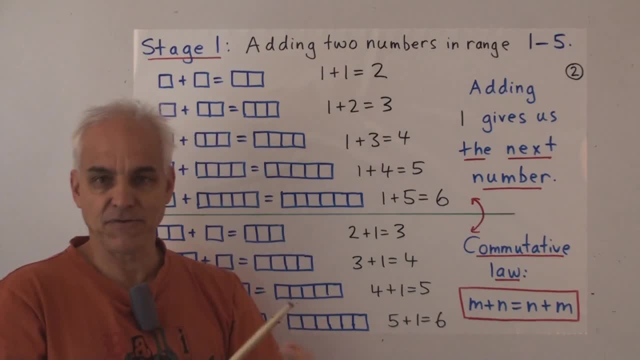 If we add one to four, we're getting the next number after four, namely five. Now there's a similar kind of opposite version of the same equations, where we add the two numbers in a different order, where we add one after the number rather than before. So 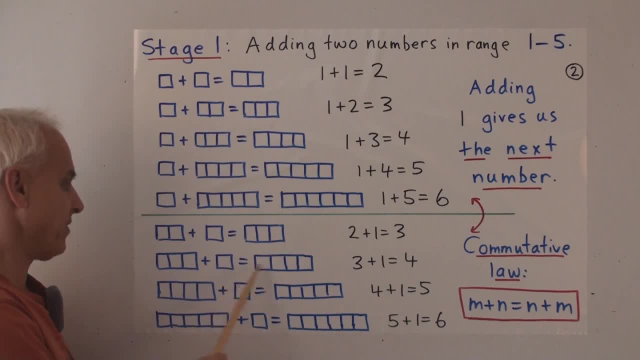 two plus one, of course, it's still three. Three plus one, it's still four. Four plus one is still five. Five plus one is six, And they're the expressions in Hindu-Arabic form. And pretty clearly, if we add one plus two, this combination, we're getting the same thing as when we add: 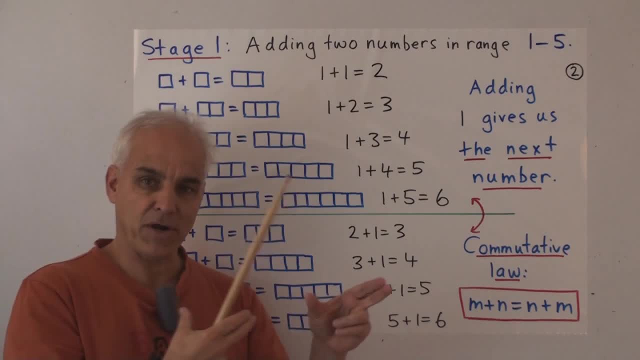 two plus one. It doesn't matter which order we're taking these two strings in. We have these two rectangles. We can either do this one together with this one, or we can interchange. in this order. The number of squares in the result is going to be the same, And that's. 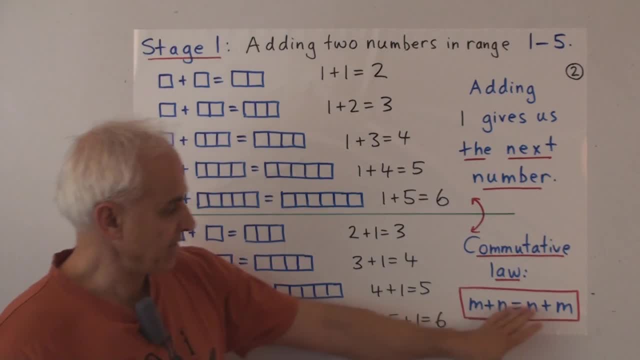 the commutative law of addition, And here's our sort of fancy expression for that. And we're going to say that m plus n equals n plus m. That's our way of saying that no matter what numbers we choose- m and n- it doesn't matter. if we add m plus n, we get. 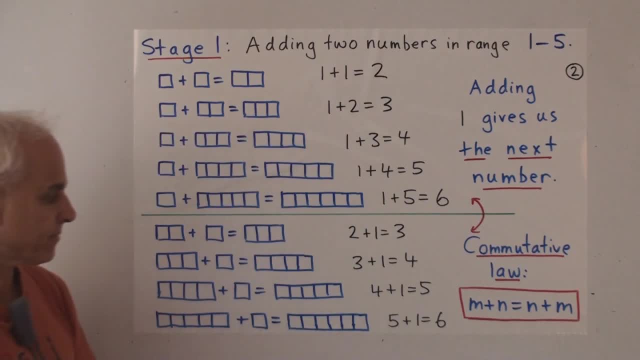 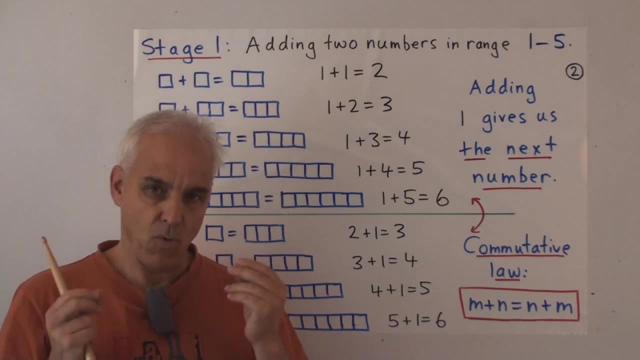 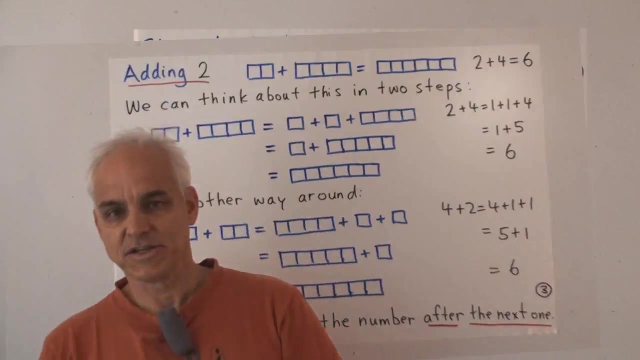 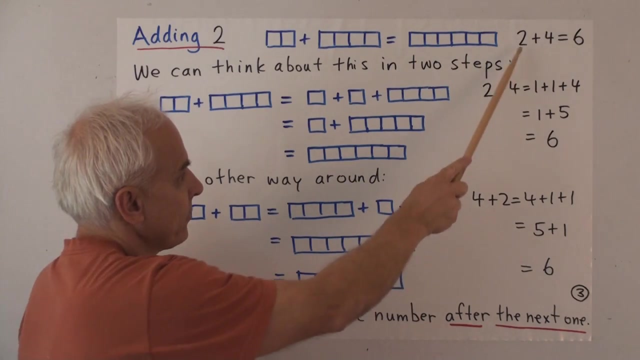 the same thing as n plus m. Alright, so those are probably the simplest kinds of addition: adding one to a number. After that we get to add two to a number. So we're going to have two. So let's consider adding two to a number. For example, two plus four equals six, Two. 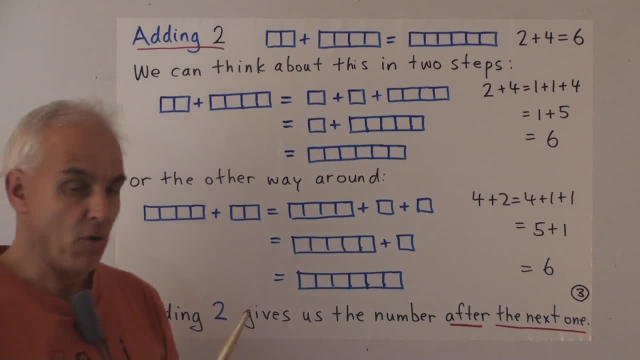 plus four equals six. If we didn't already know that, we could think about that in two steps. We could think first of all of rewriting two plus four as one plus one plus four, breaking up the two into one plus one, And then we could put these together by first combining. 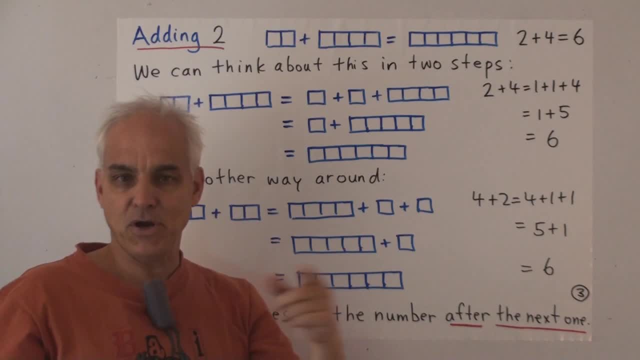 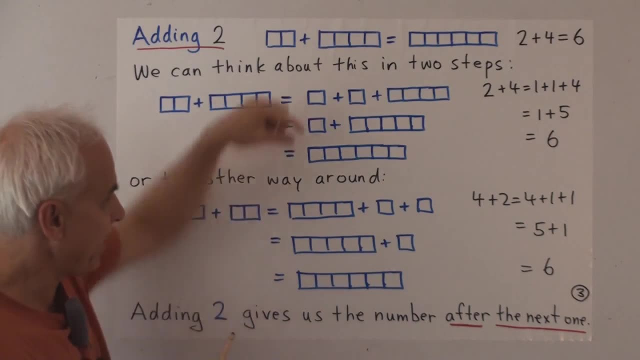 this one with that four, which we assume we already know what that is. That's from the previous slide. the next number past four, namely five, And then at the next stage we have to do exactly the same. We have to add one to that, so we're getting the next number. 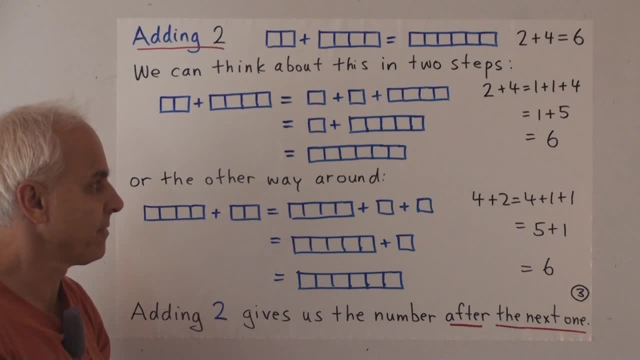 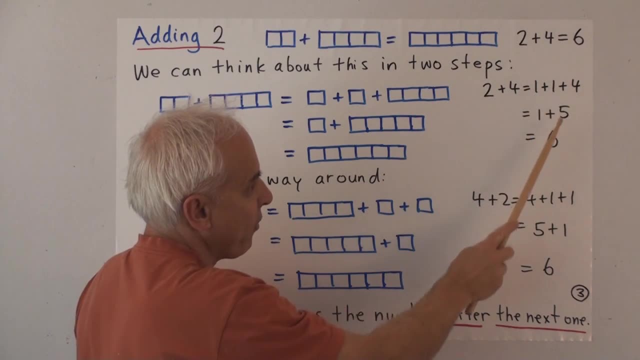 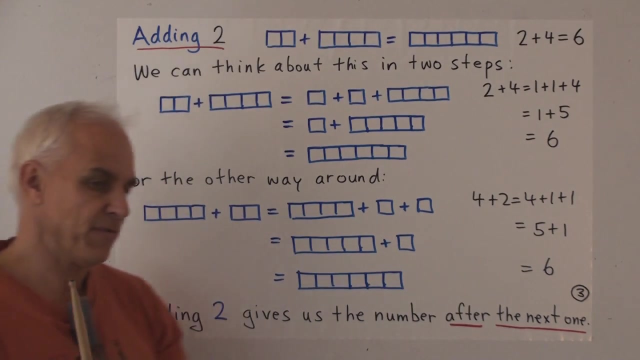 past five, which is six. So we could also say what we're doing here, we're thinking about it: two plus four is one plus one plus four, and that's the same as one plus five, And that's six. So in other words, if we know how to add one to a number, then we know how to add two to. 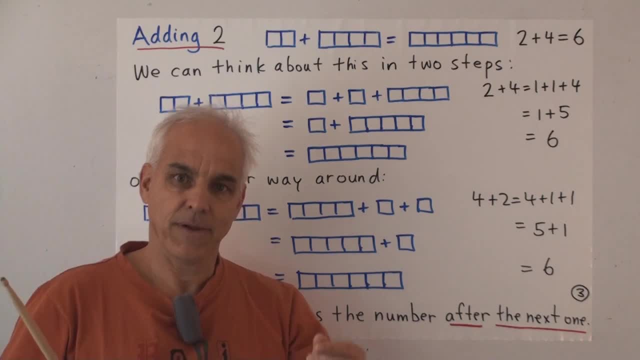 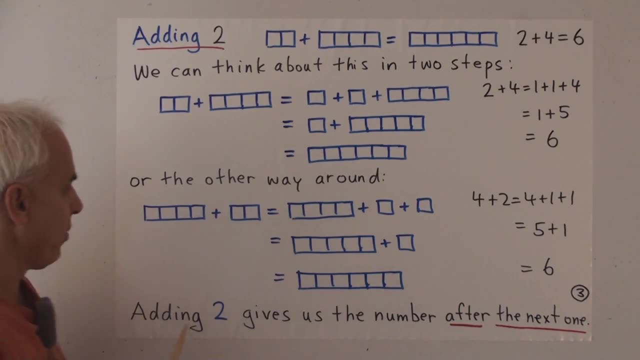 a number, We just add one and then add one again. So we add one twice. And here's the other way around, where we add two after the number rather than before. So four plus two is the same as four plus one plus one, And we can think of that as. 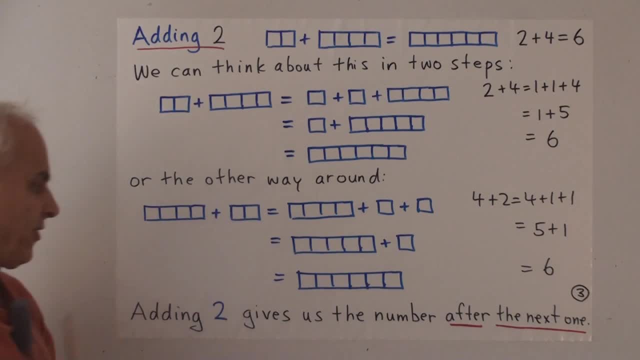 being five plus one, And that gives us then six, And a little thought shows that. another way of saying what's happening here is that adding two gives us the number after the next one. So if we add two to four, we're not getting five, but we're getting the one after that. 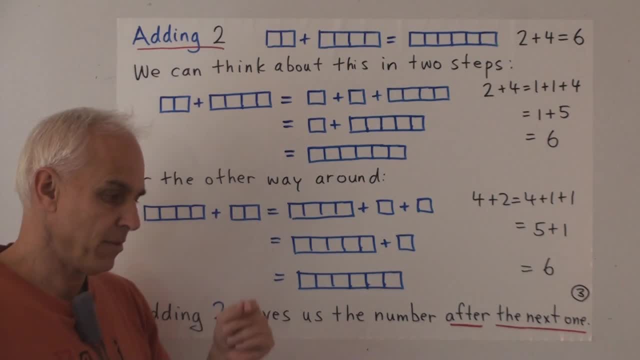 namely six. If we add two to three, we don't get four, we get rather five. If we add two to seven, we go to nine, et cetera. So first we learn how to add one, then we add two, then we extend to adding three. 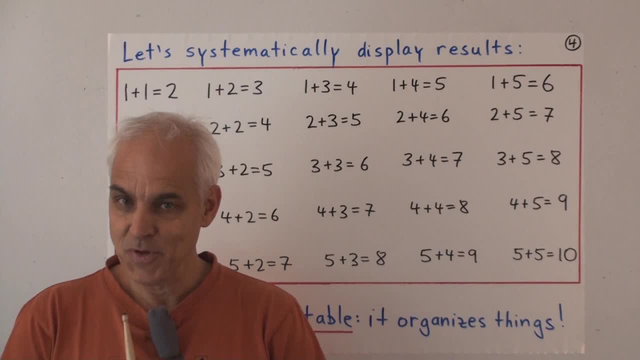 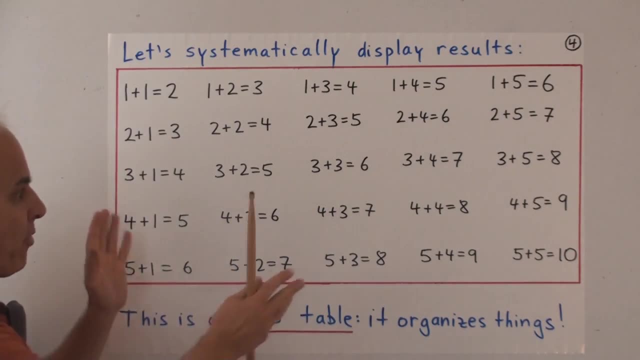 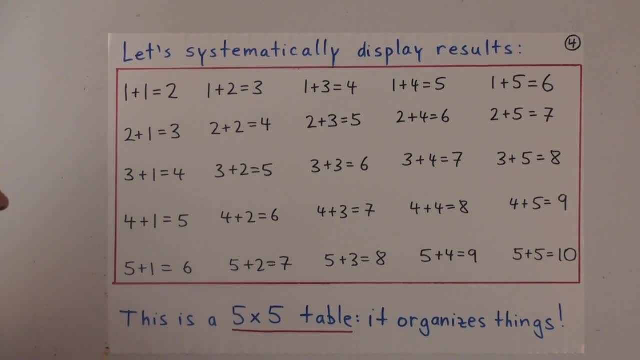 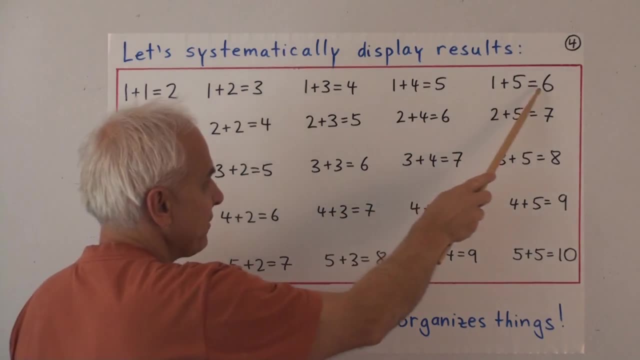 I have all the additions involving the numbers one through five. One plus one is two. One plus two is three. One plus three is four. One plus four is five. One plus five is six. And here's adding two. Two plus one is three. 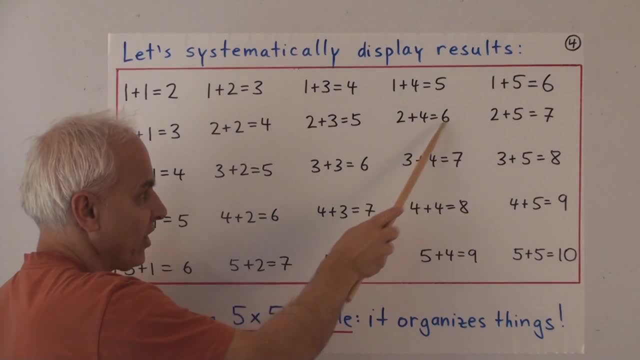 Two plus two is four. Two plus three is five. Two plus four is six. Two plus five is seven. In either case, for example, we get the number that's two past four. Three plus one is four. Three plus two is five. 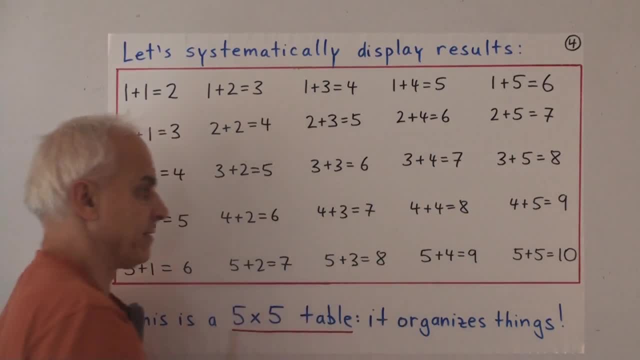 Three plus three is six. Three plus four is seven, Three plus five is eight. Four plus one is five. Four plus two equals six. Four plus three equals seven. Four plus four equals eight, Four plus five equals nine, And five plus one equals six. 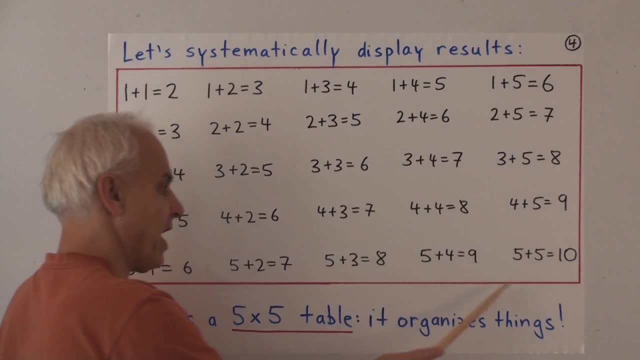 Five plus two equals seven, Five plus three equals eight, Five plus four equals nine, And five plus five equals ten. This is a table which is like a rectangle. In fact, it's a 5 by 5 table. It's got. 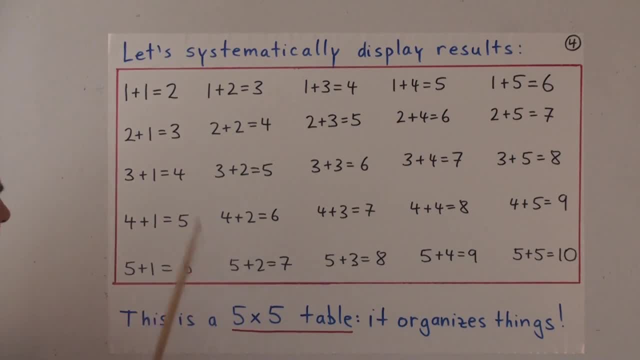 five rows and it has five columns And it's kind of a pleasant table. There's an obvious pattern If we look at the answers: here we get an answer of 2.. Here and here we get an answer of 3.. Along here we get an answer of 4's. Along this. 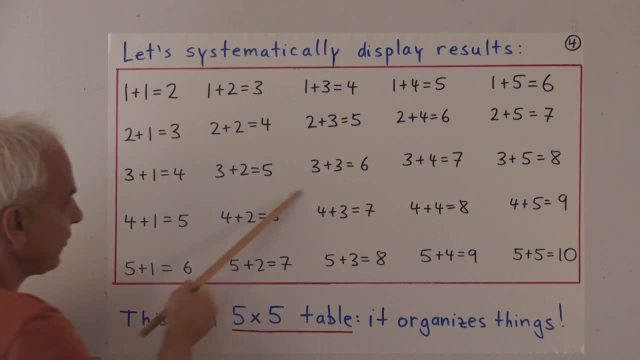 diagonal, we get an answer of 5.. Then along this diagonal we get 6's, And then along here we get 7's, Here 8,, here 9, and here 10.. It's also important to remark that there's some symmetry in 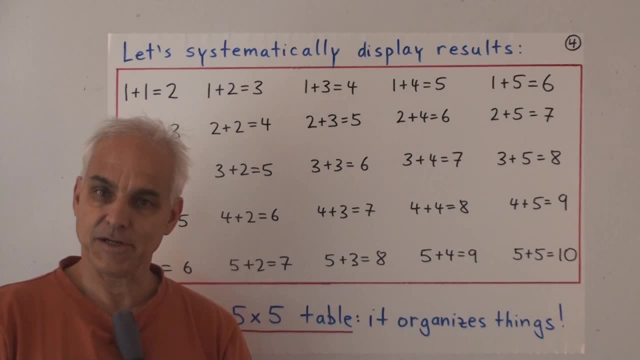 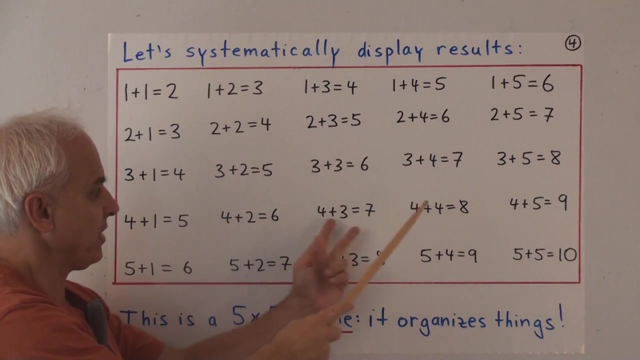 this table, which makes it in fact less difficult to memorize than it might appear, Because once you've figured out what 2 plus 4 is, then 4 plus 2 is the same. So there's a symmetry between this entry and this entry, Or between this entry and this entry. 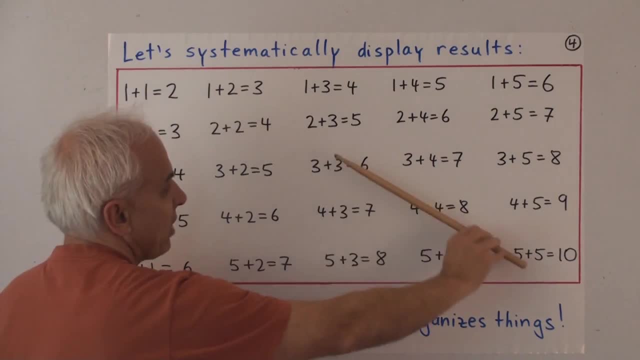 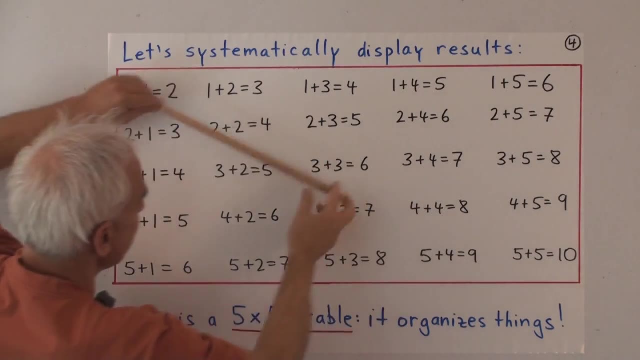 Or this entry and this entry Sort of a mirror image along this main diagonal. So in some sense we can say that what we really only need to remember is everything on that diagonal and say above it, Or everything on that diagonal and below it, The commutative law takes care of the. 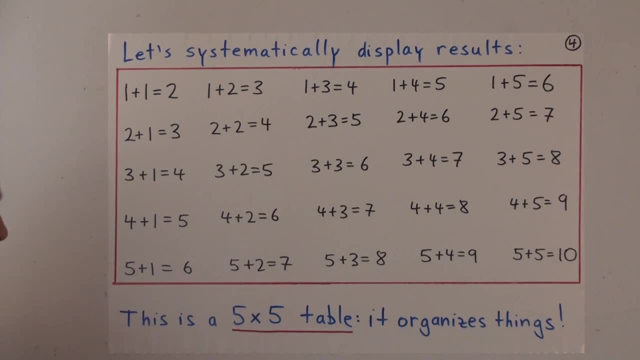 other ones. Now, it's the fact that young people have to learn this table one way or the other, And I'm not going to make definitive statements about how young people should learn these things. I think that's best left to primary school educators to figure out. I'm just pointing out that this is a 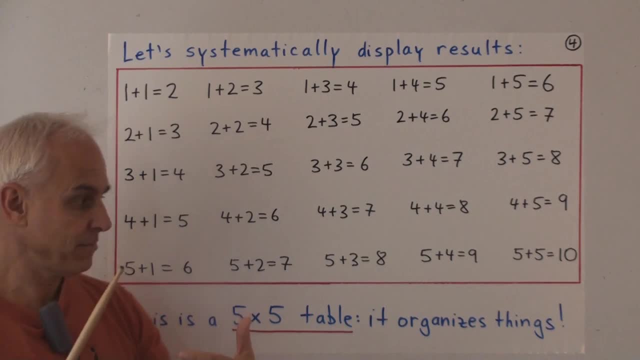 a very important preliminary understanding that all students of mathematics have to have to make progress in arithmetic and consequently in mathematics. Let's rewrite this table in a little bit, I think, more attractive way. There's a little bit too much in this table and it's possible to make it. 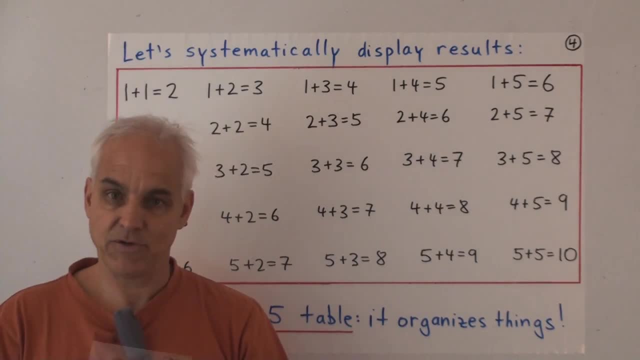 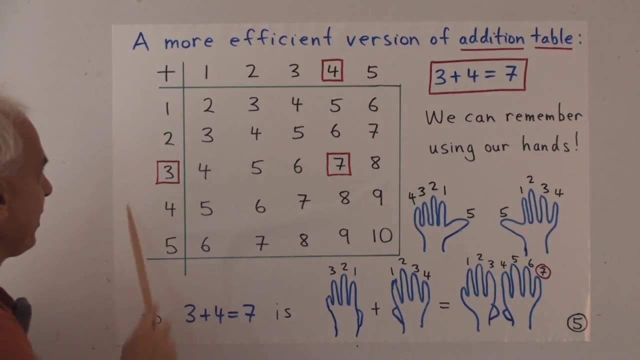 more efficient and therefore perhaps easier to remember. So here is this more efficient pared-down version of this addition table. Here it is right here. So let's have a good look at this. make sure we understand what this is telling us. First of all, this is a table for addition, So this little sign that I'm 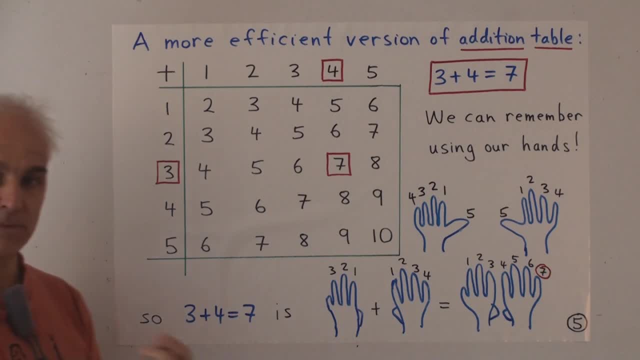 putting here makes it clear that we're talking about addition, not multiplication. Later on, we'll have a similar kind of table for multiplication, which will be a little bit more complicated. This is a pretty simple table, as you can see, because the pattern is reasonably clear. 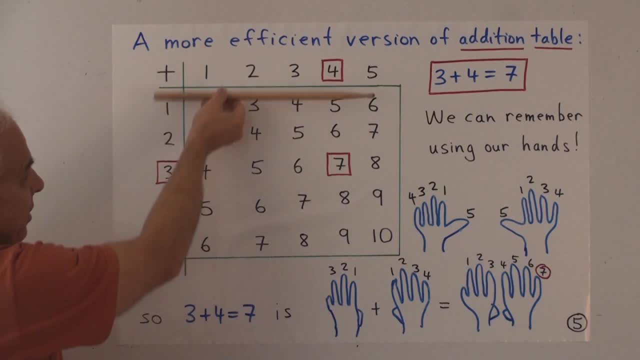 What is the definition of multiplication? What is the definition of multiplication involved here? Well, we have some lines here separating numbers 1,, 2,, 3,, 4, 5 along here, and numbers 1,, 2,, 3,, 4, 5 along here, with the main body of the table And the 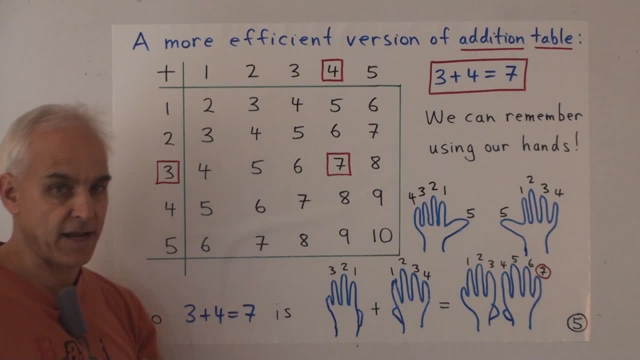 way we read this is, if we want to add two numbers- let's say 3 and 4, we go down this first column till we get to the first number 3.. We go along this top row till we get to the second number 4.. So we're adding 3 plus 4.. We'd like to know. 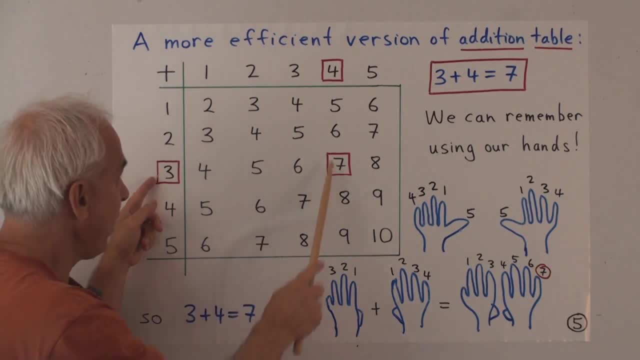 what that is. Then we go along this row and down this column to where they meet, and the entry here is the answer of what is 3 plus 4.. So 3 plus 4 is 7.. Let's do some more. 4 plus 2 is 6.. 5 plus 3 is 7.. 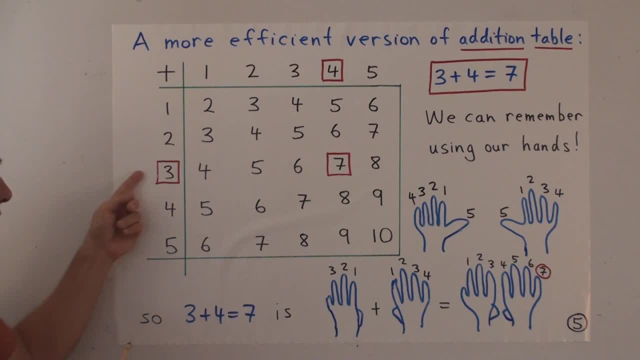 3 is 8.. 3 plus 5 would be 3 plus 5.. That's also 8.. So the symmetry that we talked about before, the commutative law symmetry, is telling us that this table is symmetric. if we reflect along this diagonal, This 7 is the same as that. That. 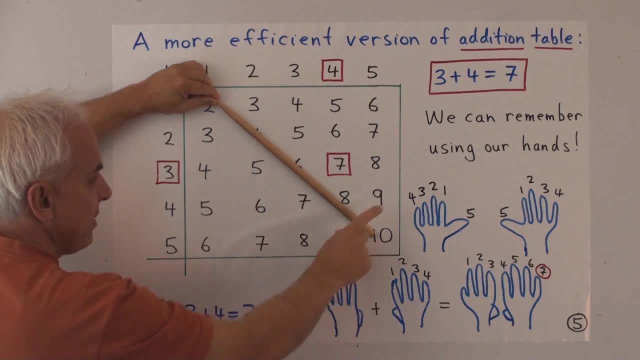 5 is the same as that, That 6 is the same as that, 7 is the same as that, That 9 is the same as that. Of course, it's pretty easy to see here that there's a nice pattern, because along every row 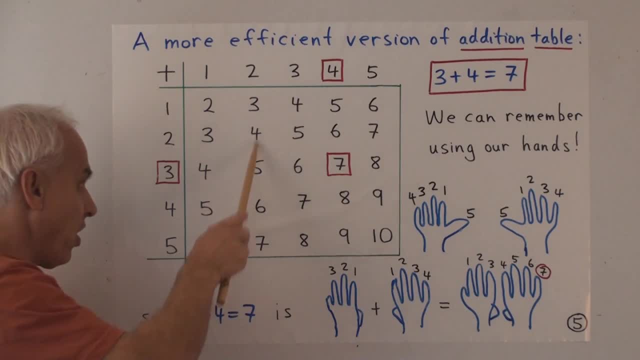 we're just going up one at a time, Down every column. we're just going up one at a time And along these sort of cross diagonals we have 3s, 4s, 5s, 6s, 7s, 8s, 9s, 10s. 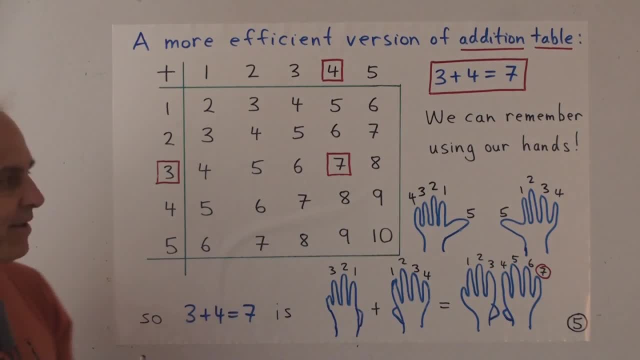 So if you forgot this table, it wouldn't be too hard, by starting out with 1 plus 1 is 2, to reasonably quickly draw the rest of the table. Okay, it's not a mystery of how to construct this table. 1 plus 1 is 2.. That's the first and the most simplest addition, And 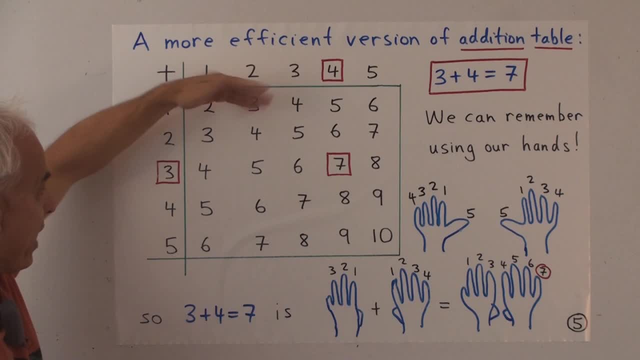 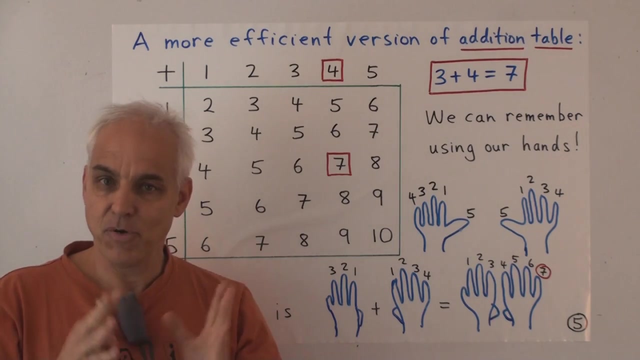 everything else is built up from that by moving sequentially one up as we go along the row or column. Okay, so students of course have to learn this And they have to find some way of of putting that in their long-term memory. That's a very important job for. 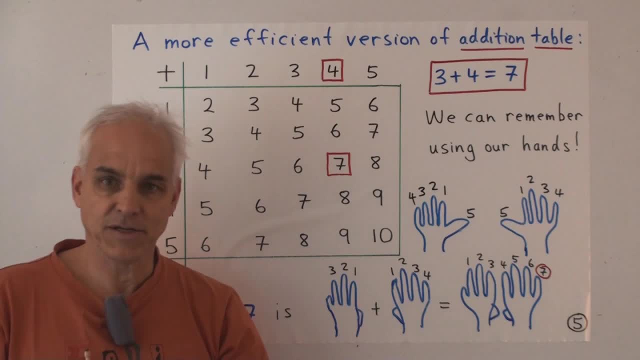 teachers and for parents, And you might use cue cards and you might use lots of examples. You might use your hands, And I'd like to point out the usefulness of thinking about our hands as a way of encoding or perhaps allowing us to calculate such simple sums, or especially for young people, if they've 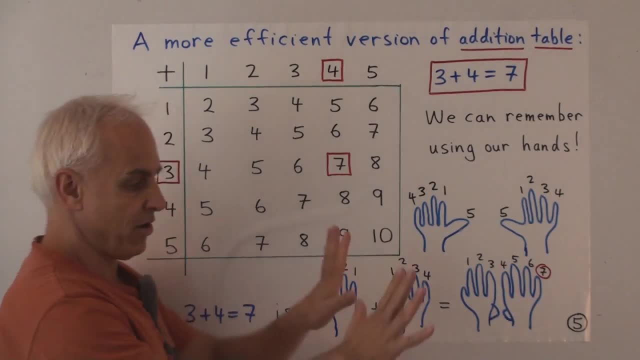 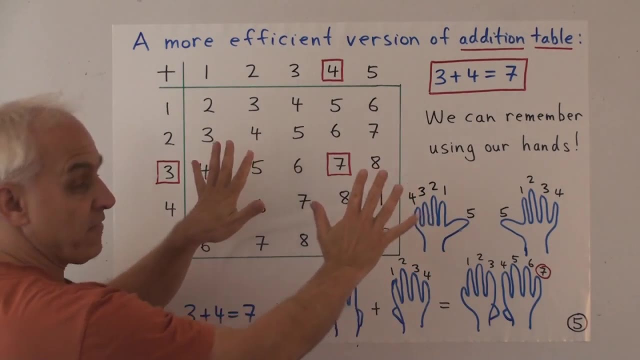 forgotten it. So here are my hands, and left hand and right hand. That's what's represented here And we can use our our hands or the fingers on our hands to do some counting. There's different ways of doing this. Different cultures have. 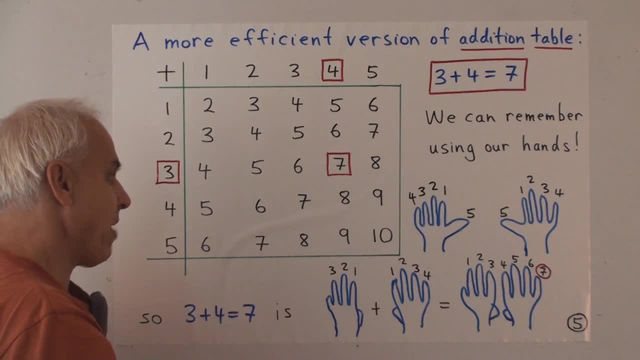 different ways of representing the various numbers. Probably I think it's simplest if, if we say: use the left hand index finger to be number one, And then that combination is 2., That combination is 3., And that combination is 4.. And then when we add the thumb we get 5.. And on the 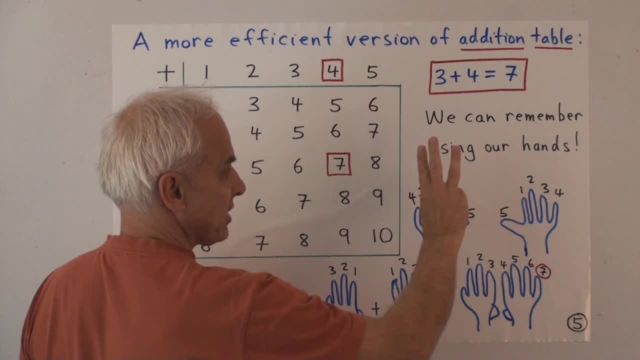 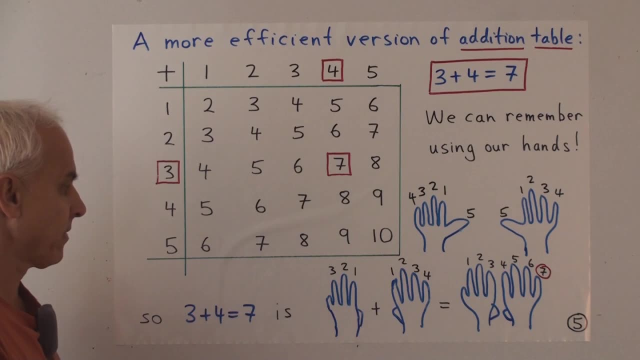 the other hand, too, we'll represent this to be 1,, this is 2,, this is 3,, this is 4, and this is 5.. So we're only dealing with the numbers from 1 to 5 at this stage. So 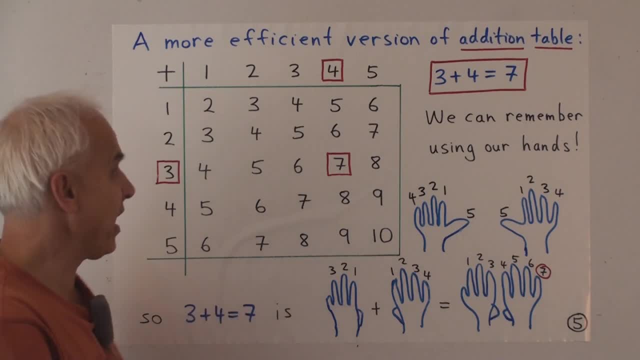 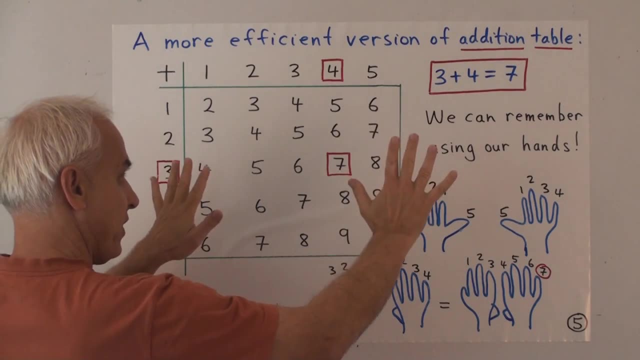 for example, if the student wanted to use his hands to calculate 3 plus 4,, what they could do is they could use this hand for the first number 3, and this hand for the second number four, and then they could use their fingers. How would that work? 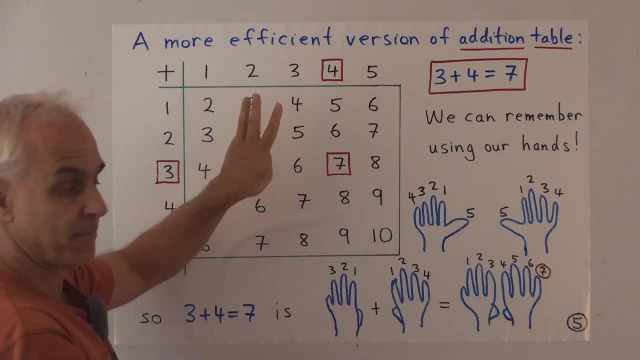 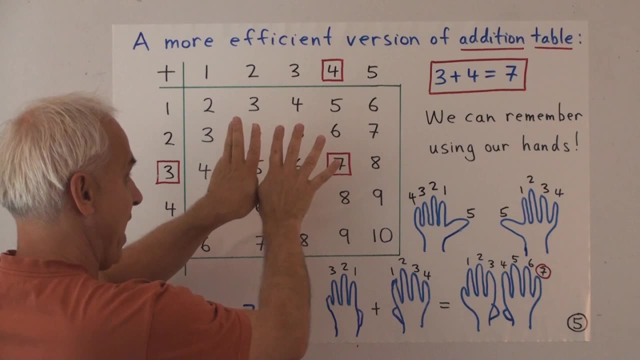 Well, the number three represented on this hand would be that The number four represented in this hand would be that: So there's three and there's four, and the student can think about adding them, is just putting them together. Well, then you have to count. How many is that? 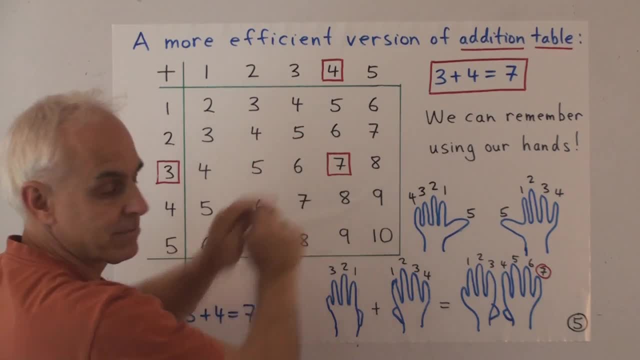 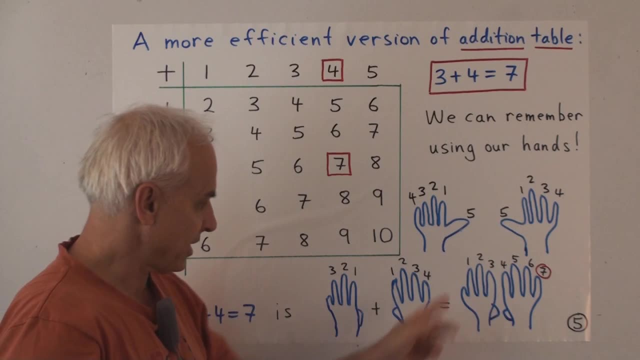 One, two, three, four, five, six, seven. So three plus four is seven. This represents the final counting. after you put them together, The student can count them off one by one till they get to seven. A variant on that would be to say: I will start with three. 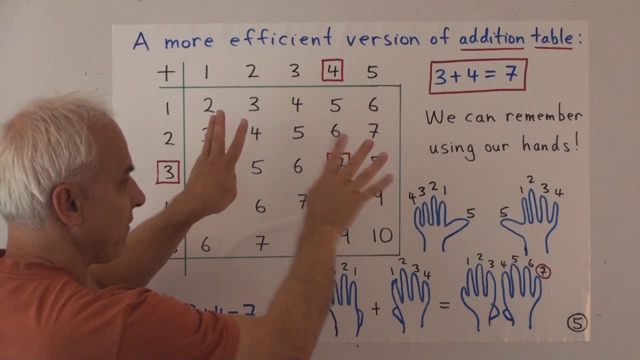 and then we'll add four. So adding that four means we get four and then five and then six and then seven. In other words, we can assume that we already know we have three, because that's the first number, and then we're adding one more. 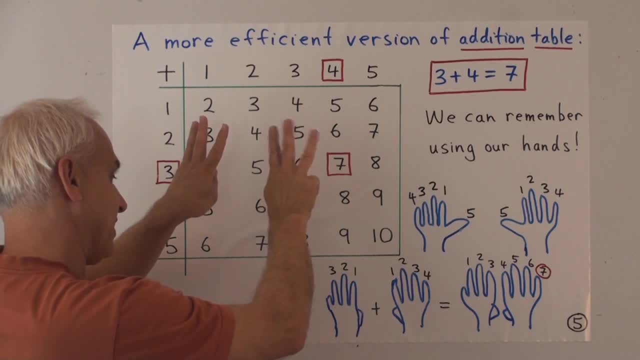 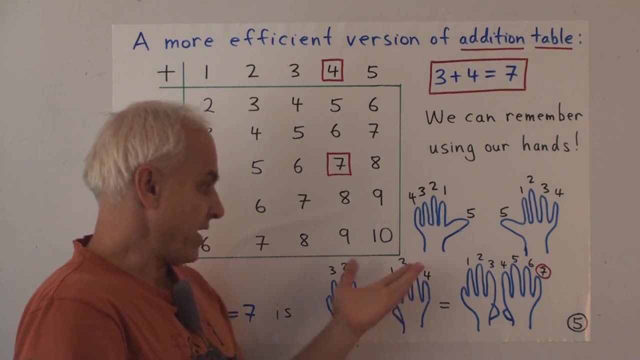 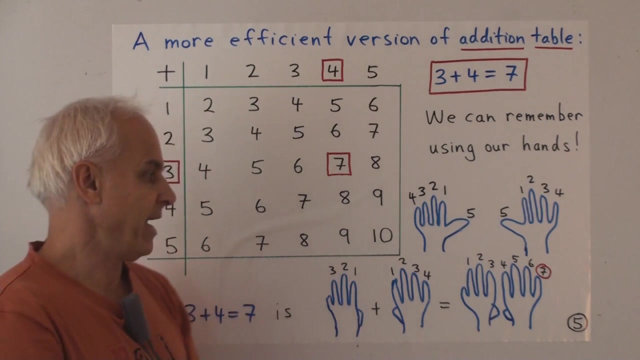 to get four, another one more to get five, and then one more to get six, and then a fourth, one more to get seven. So it's quite natural, Of course. this is where our number system arose, by fingers of the hands, and it's quite reasonable for students. 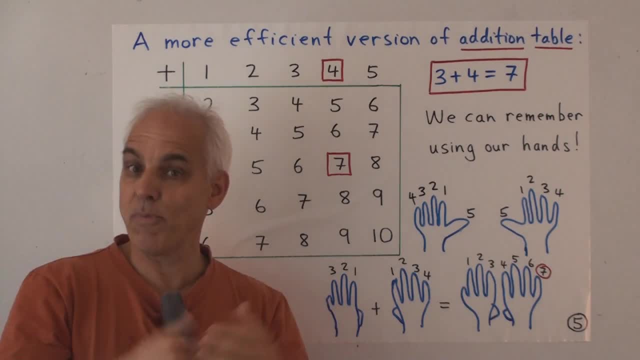 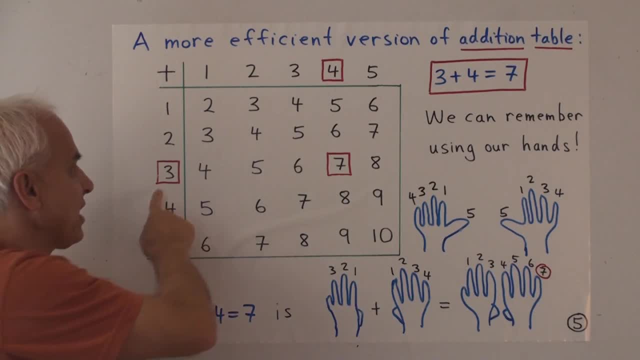 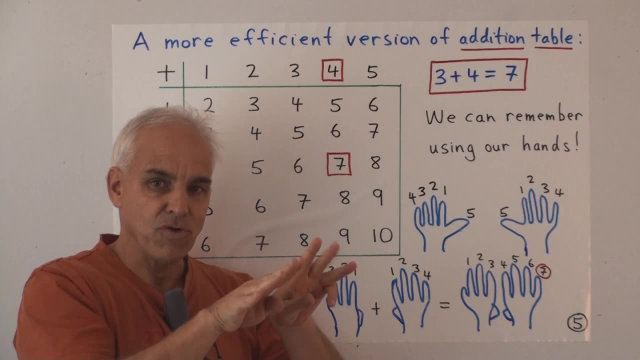 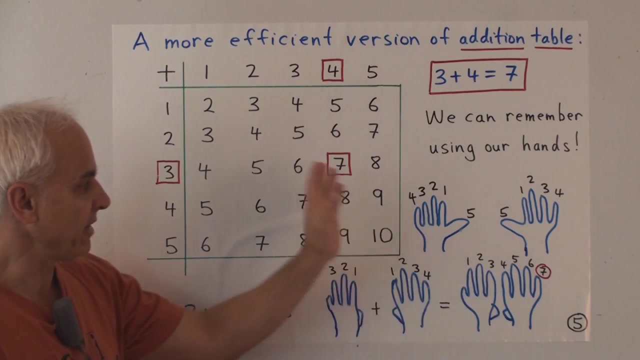 And think symbolically. So ultimately, when a student sees three plus four, they should be able to say seven without in their minds or under the desk using their fingers. So this is a preliminary kind of business, but later on we just want to memorize this. 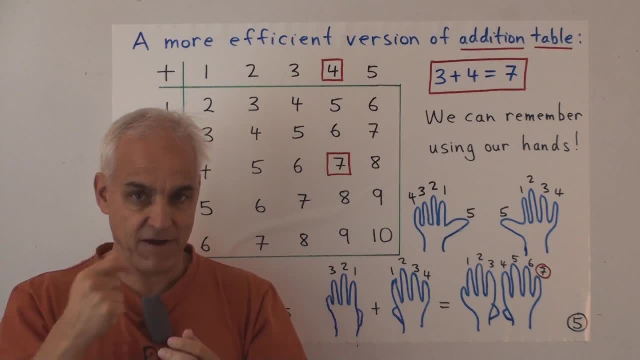 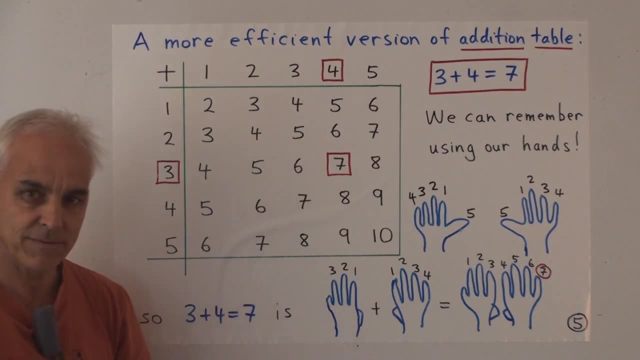 table and have it solidly in there so that they can very, very quickly tell us the result of the sum of any two numbers plus five, it's nine. Very quick. Probably it's not bad even just repetition If a student has 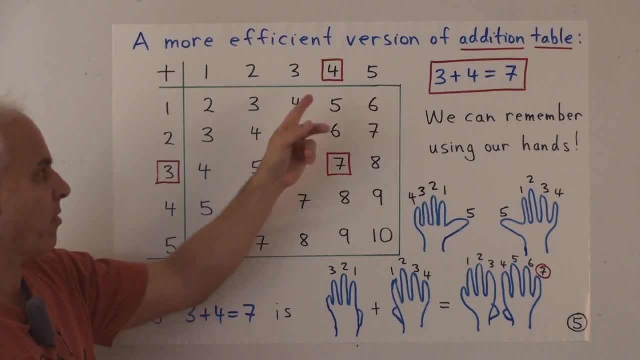 to read this table. one plus one is two, one plus two is three, one plus three is four. one plus four is five. one plus five is six. If you read that table, simply do that a couple of times a day probably- it doesn't take too many weeks before those facts are solidified into the long-term. 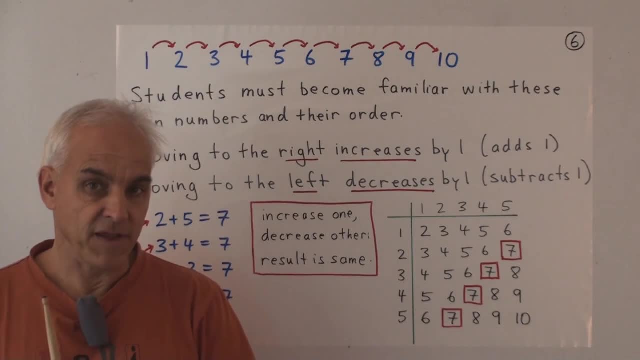 memory. So all the numbers involved in this five by five addition table are all in the range of our basic first ten numbers, from one to ten, And as the student becomes familiar with addition they should also become more and more familiar with these ten numbers and their relative positions. 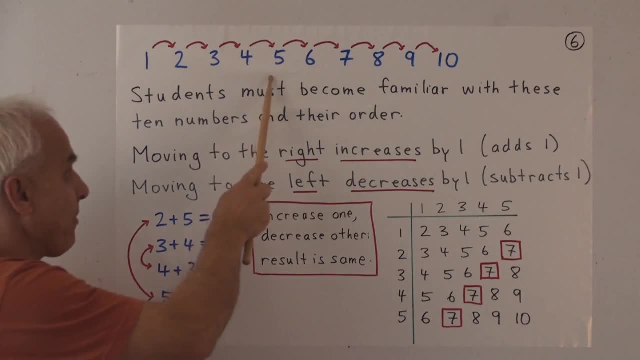 So by relative position I mean that, given any number, they should know which is the next number. They should know which is the next number. They should know which is the next number. They should know which is the previous number. It should not be too hard for them to figure. 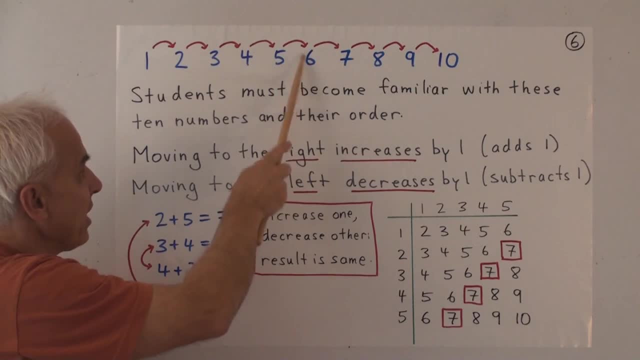 out what's the number that's after the next number or what's the number that's before the previous number. So, of course, moving to the right in this list increases by one or, if you like, adds one. Going from here to here is adding one From here to here is. 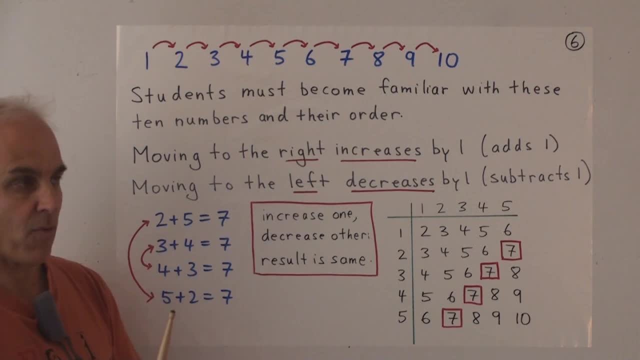 adding one While moving to the left, decreases by one. Well, that's subtracting by one. So subtraction which we haven't talked about, but it's subtracting one, It's taking one away. So here's our addition table again, and I've just pointed out this cross diagonal here, the various 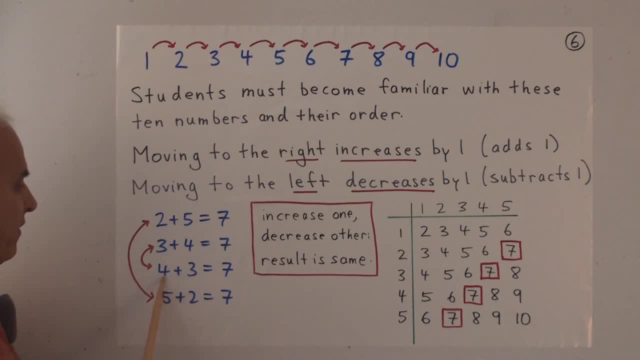 sevens, which are the result of two plus five, three plus four, four plus three, five plus two. Those are all the ways of getting seven by adding two numbers, And it's useful for students to be aware that the number that's after the first number is the number that's after the second number. 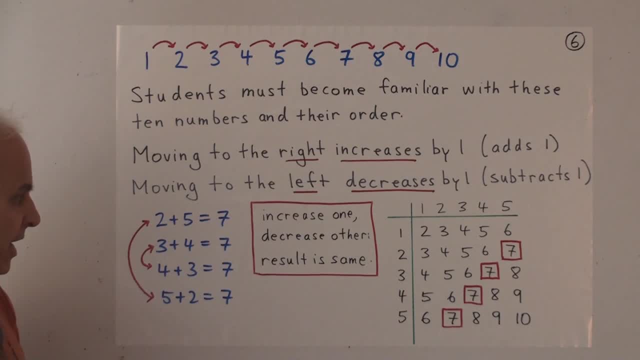 If you have two numbers and you know what the answer is, that if you decrease or increase one of the numbers and simultaneously decrease the other, then the result is the same. So if you know what two plus five is, it's seven. then if you increase the two by one and simultaneously you decrease the 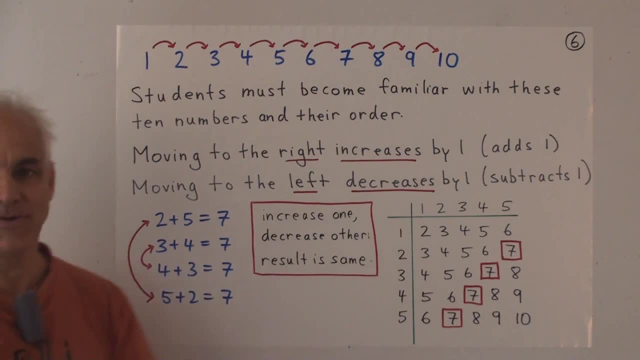 five by one, then you get three plus four. That's also got to be seven. So that's a way of helping organize our understanding of the number. So if you have two numbers and you know what the answer is, you can just add a number to the addition table. So, for example, let's have a look at two plus three. 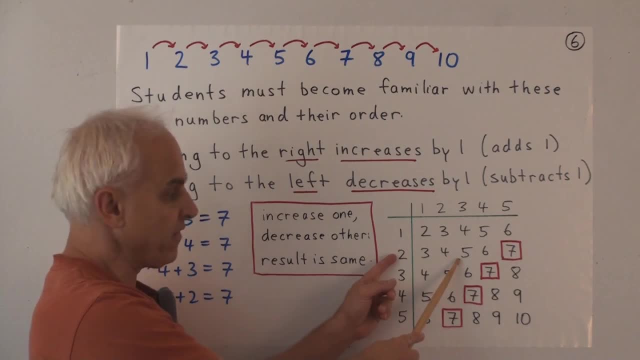 There's two plus three is five. If I happen to increase one of the two numbers, suppose I increase the two to three. So instead of having two plus three I have three plus three. So I've increased that number by one. then the result is also increased by one. Or if I increase the three by 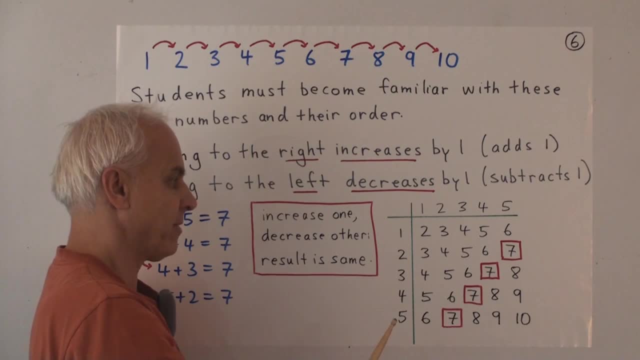 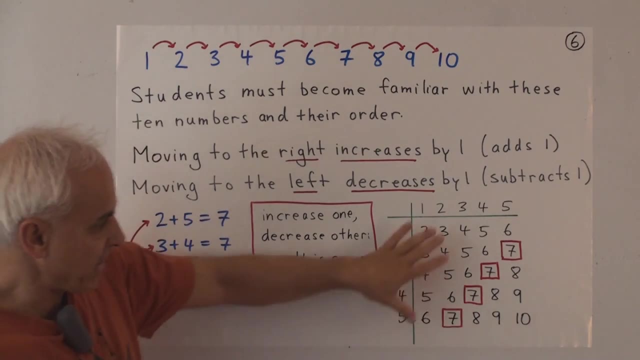 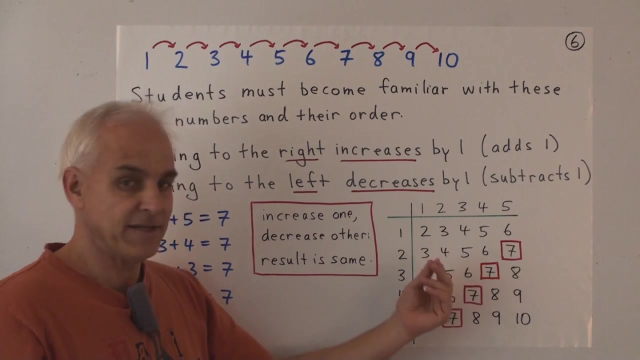 one, then I also increase the answer by one. So if two plus three is five, then the result is also five. then two plus four is six. So students should get a sense of the interconnectedness of this table, that adjacent entries have a direct and easy to understand relation to the entry that you. 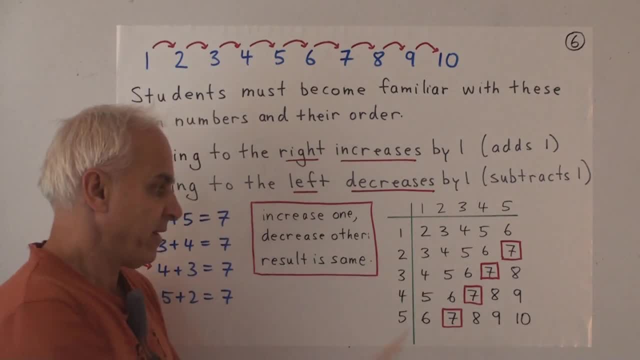 started with. If you move one of these numbers up, then the answer moves up by the same corresponding amount. If you move one of these numbers up or perhaps down, then the answer moves up or down a corresponding amount. So it's good that students get a really varied understanding of this. that 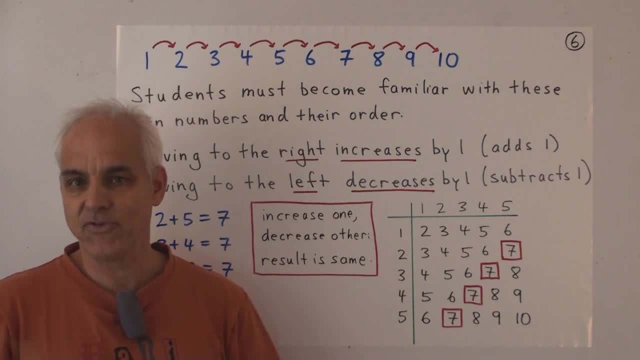 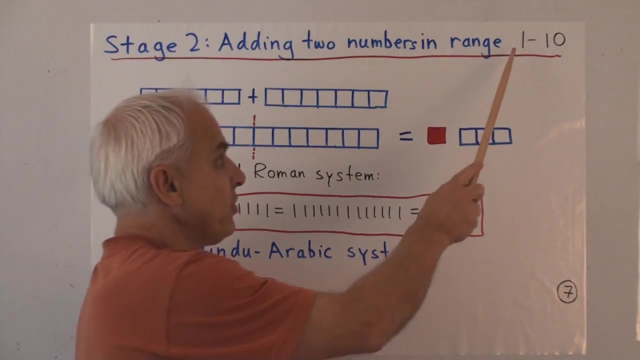 they explore this with many different examples and many different problems that can illustrate various aspects of this. It's the solid basic understanding that underlies addition numbers from one to five. So now let's move to stage two of addition, where we extend the range that we're considering to numbers between one and ten. So how do we add two numbers? 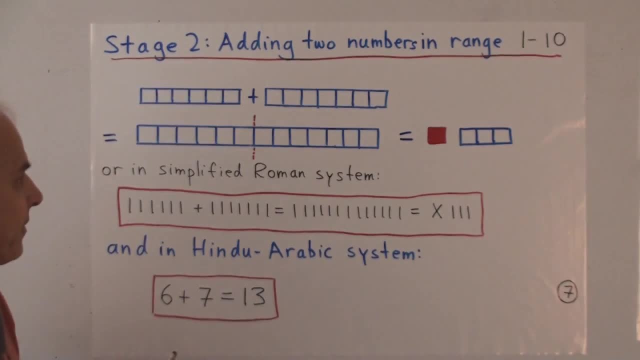 between one and ten. And how do we teach young people about that? Well, this is the kind of situation we're talking about. We have two numbers perhaps, like this one and this one, This one's six, this is seven. When we add them, we get this number here, And I remind you that the idea 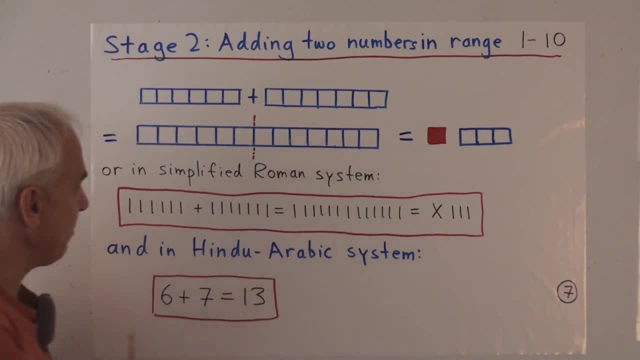 to simplify our expression for such a longish number is to peel off a ten, One, two, three, four, five, six, seven, eight, nine, ten, And represent that ten, say by that one red square, And then there will be three left over. So we end. 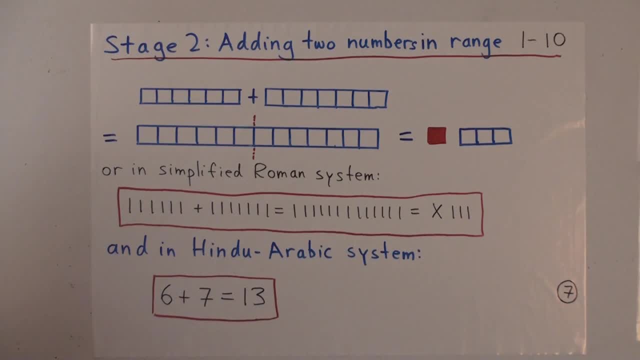 up with ten as well as three. In the simplified Roman system, this would be represented by having six there, seven there, and there is our ten, three And, of course, in Hindu-Arabic system we have six plus seven equals thirteen. Thirteen is the usual number for this Roman expression. 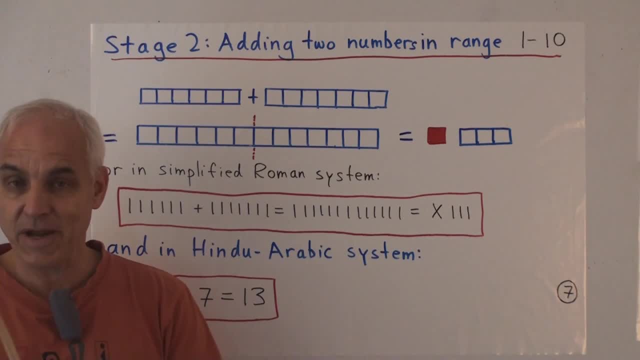 Of course, now we must extend the range of the numbers that we're considering from not just one to ten, but one up to, in fact, twenty, Because those are the possibilities that we can get if we take two numbers in this range and add them. So a preliminary to this kind of addition is to have 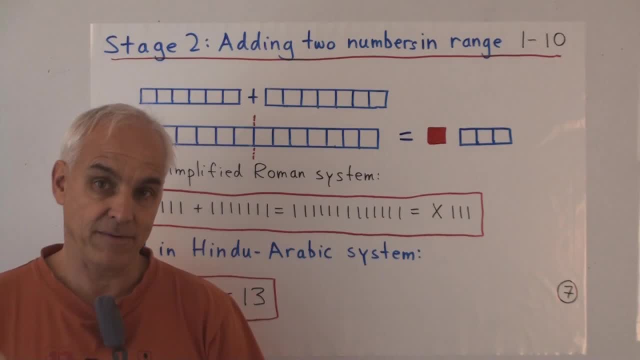 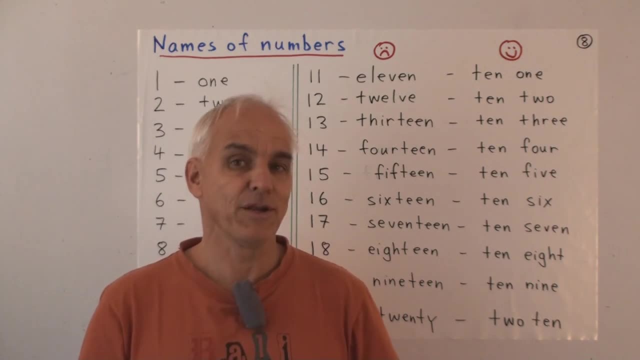 consistent names for the numbers Bigger than ten, or say between ten and twenty. And now we come to an interesting but somewhat delicate issue, that is having to do with the names for numbers. We have our symbols for numbers: the Hindu-Arabic. 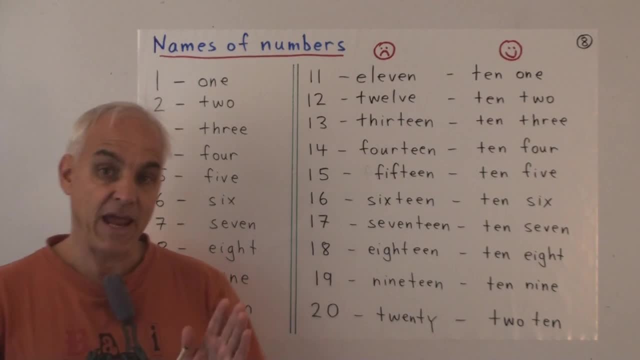 symbols, but so far we only have names for essentially the first ten of them. What about the names for higher numbers, Say the ones between ten and up to twenty? Unfortunately, our names for these numbers, and in fact our naming system in general, is rather haphazard and illogical in many places. This is a problem with the 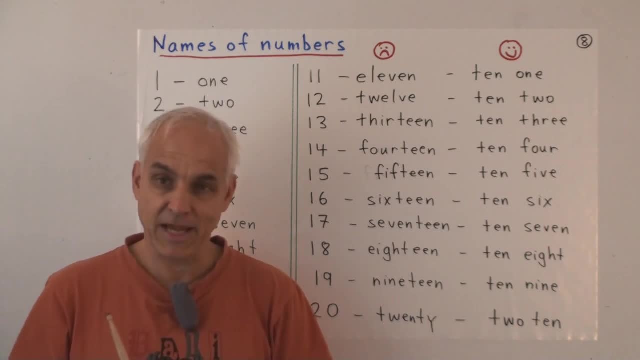 English names for numbers and doesn't necessarily extend to other languages. Other languages also have problems, But some languages deal with this challenge much more efficiently and effectively, And that means that students in these other languages- and I'm thinking of Asian languages here- they have a great advantage when it comes to learning arithmetic. 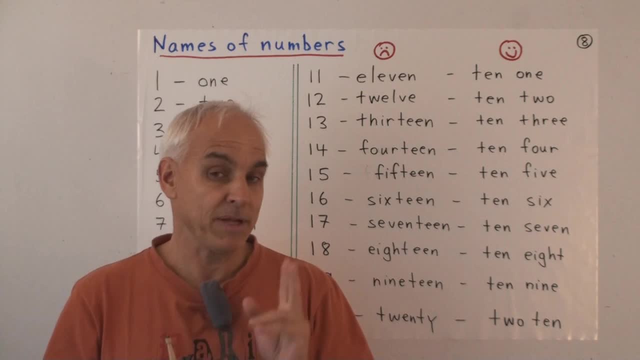 I think this point is not perhaps properly understood and properly acknowledged by educators. To a certain extent, there's nothing, it seems, that we can do about it, because the names for our numbers are so entrenched in our history that we can't. 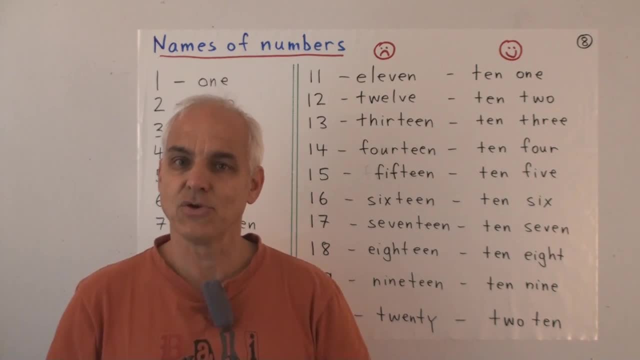 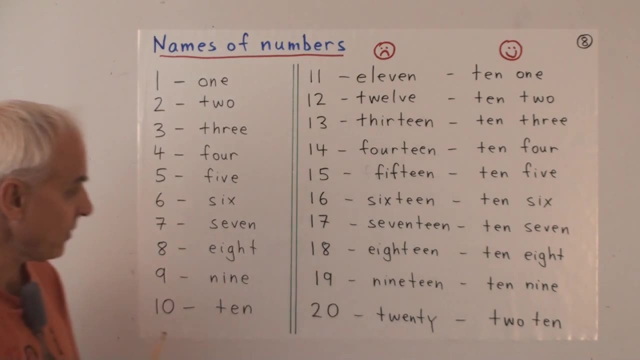 use them in our system. Nevertheless, if there is a weakness, it is good to acknowledge it, even if we are not currently in a position to overcome it. So our names for these numbers in English are 1, 2,, 3,, 4,, 5, 6,, 7,, 8,, 9,, 10.. And that's not a bad naming system. It's not. 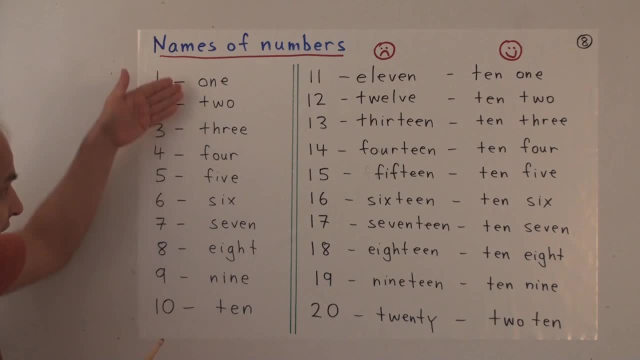 particularly good, but I don't think it's particularly bad. There's clearly something arbitrary about those names. The main thing that we want these names to have is that they be recognizably distinct, So that there's little possible confusion between one and the other, And the other thing that we would like them to be is to be relatively short- One syllable if. 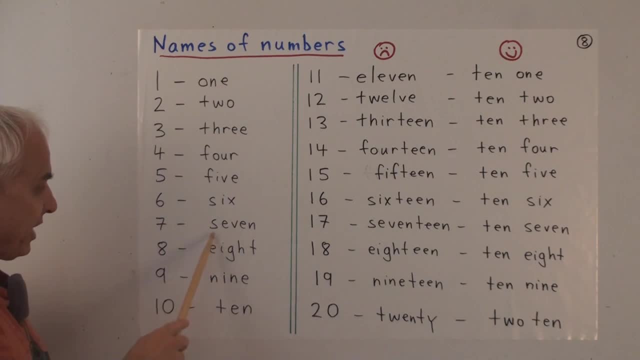 possible. Now, these are all one syllable words with the exception of seven, which unfortunately is a two syllable word, and it does introduce a little bit of additional time time time required to express numbers that involve seven. Unfortunately, the problems with 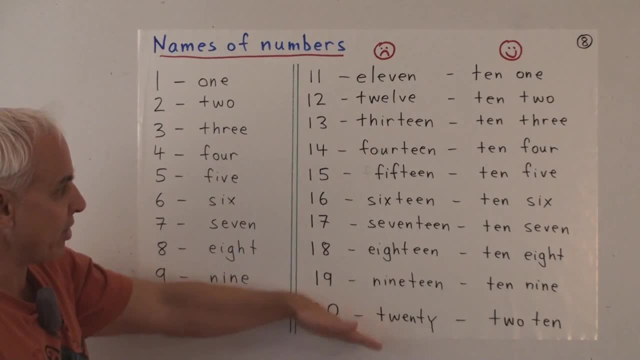 our naming are much greater when we look at these range of numbers, The numbers that we usually call 11,, 12,, 13,, 14,, 15,, 16,, 17,, 18,, 19, 20.. Now, if you're any person, 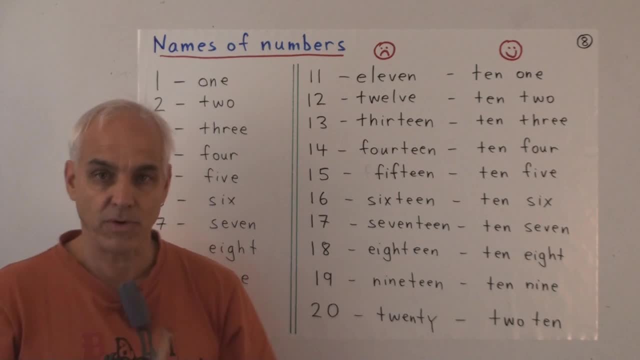 over the age of you know 10 in the English-speaking world, you will know these words and you will be very familiar with them. However, if you're a very young person, it takes some time to learn these words and it's not. 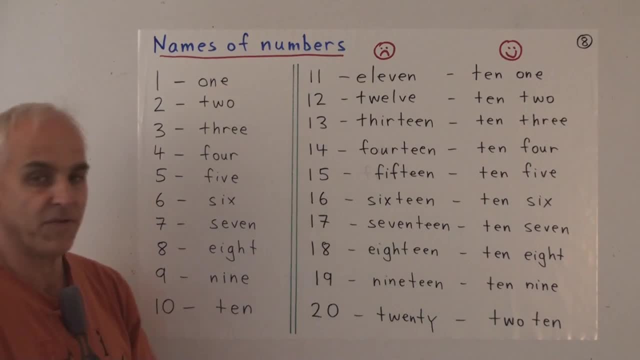 particularly logical the pattern of the names that we're using. The words are rather long and their connections with the symbols are a little bit arbitrary, somewhat tenuous. Okay, we can recognize. the 12 sounds like a two, The 13 sounds like a three, There's a four and 14. There's almost a five in 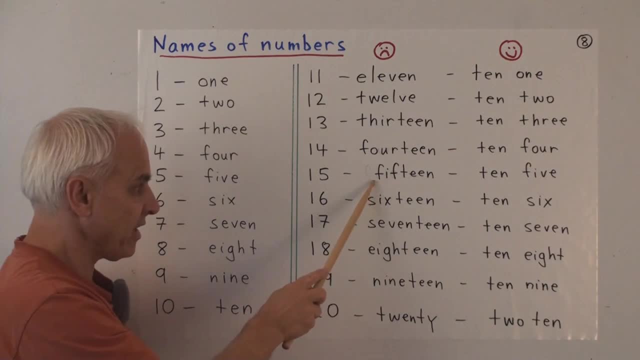 there, but it's spelled differently, although sometimes it's still spelled F-I-V-E-T-E-E-N. There's a six, obviously, there a seven, there we see an eight, there a nine, there a twenty. that seems to come out of the blue. As for the tens, well, the ten is sort of. 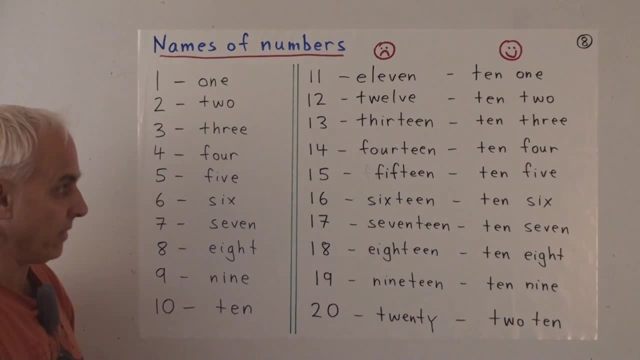 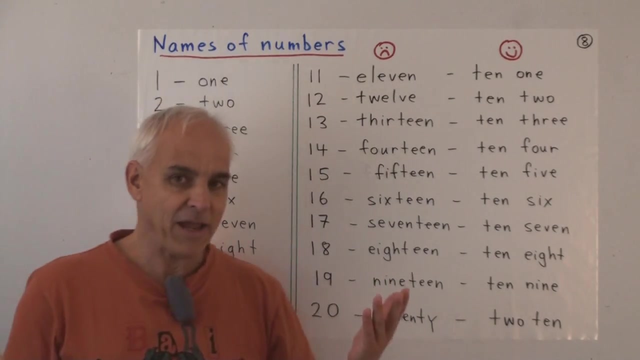 represented by this elongated ten which is now a teen, for some strange reason, and that only starts with 13. And 12 and 11 are somewhat odd. Now, the adults among us are so used to this we don't bat an eye. We say, well, that's just the way life is. Well, here is a proposed 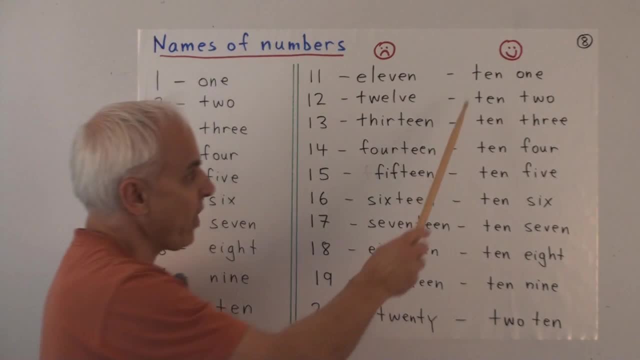 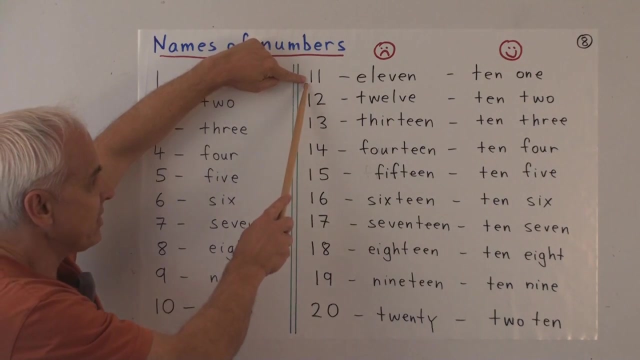 alternate system. This is another way that we might think about naming these numbers and it has a lot to recommend it, this alternate way. So we are going to look at this Logically. looking at this, this is 110 and 11, which is encoded. 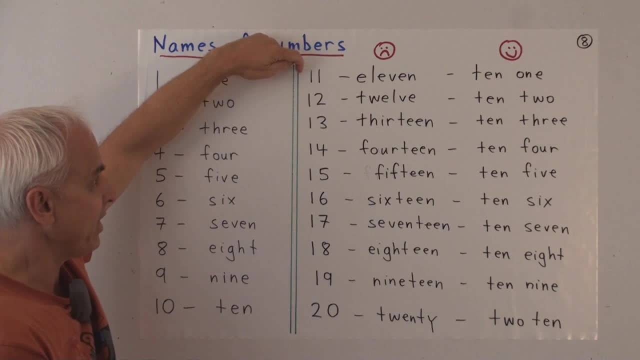 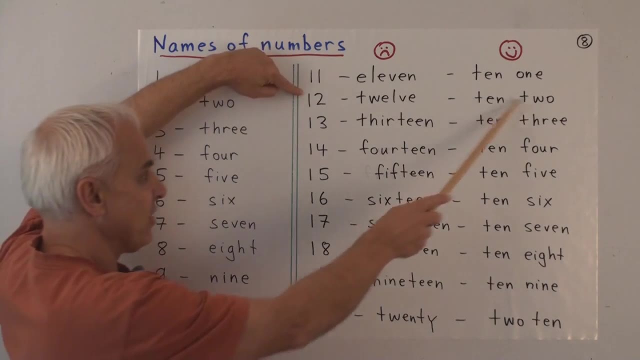 very efficiently by the two words 10-1,, reading left to right. Here is 10 and 2,, so a good name for this number would be 10-2.. Then here is 10-3,, here is 10-4, and the pattern is: 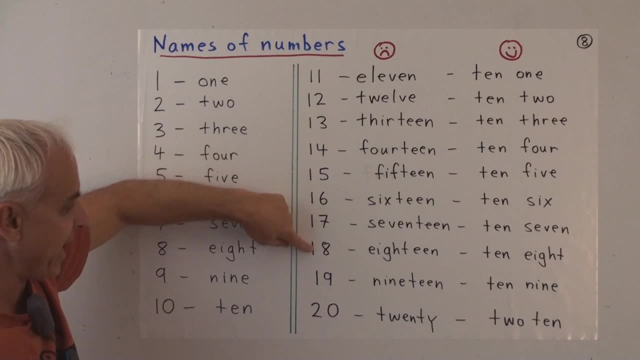 completely obvious: 10-5, 10-6,, 10-7,, 10-8,, 10-9, until this number. What's this number? 10-3.. What do we see here? We see two 10s and zero 1s, so we don't need to include the 1s. we. 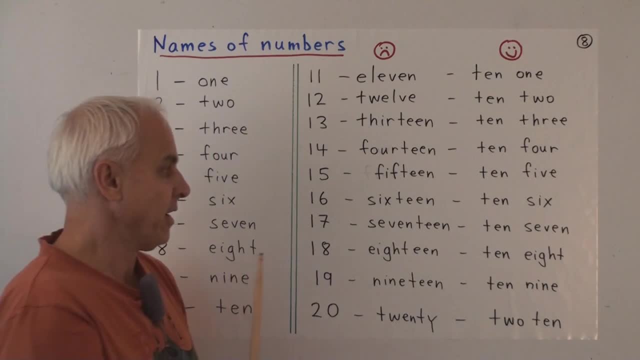 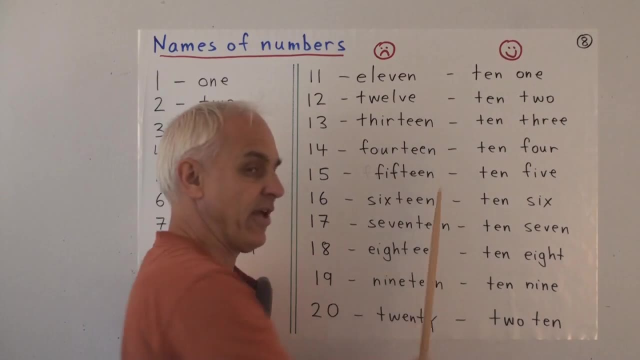 just say 2-10.. So am I seriously proposing that we change from this traditional naming system to this much more logical, sensible one? Well, not altogether, But I am proposing it in a small way, I am suggesting that you think about it, You think about the possible. 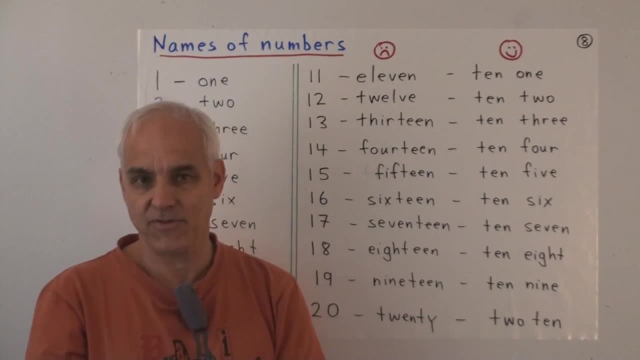 advantages in having a naming system that's like this. It would make the job of learning arithmetic for young people much simpler And the idea that mathematics is a logical enterprise, that it's not dependent on a lot of ad hoc things that you have to memorize. 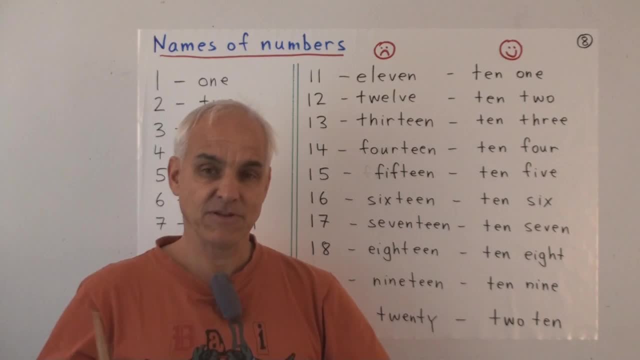 It instills that idea more firmly into young people's minds and gives them confidence that they can understand patterns And learn patterns and trust them. I think the education of young people in Western countries in the current time would be vastly improved if somehow we could miraculously take our 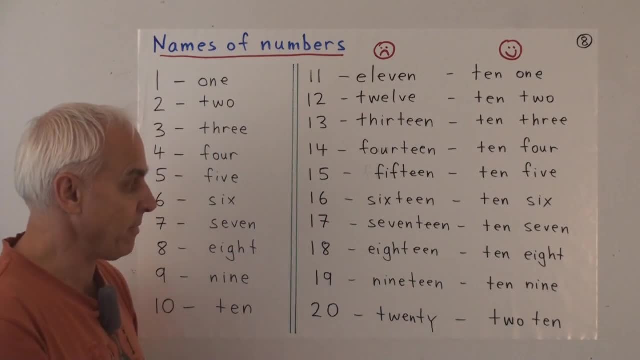 magic wand and replace usage of these names with usage of these names. So I wanted to point that out. Maybe people can give some thought to this suggestion And, just for fun, I might actually try to use these new simplified names instead of these ones. You'll easily, of course, be. 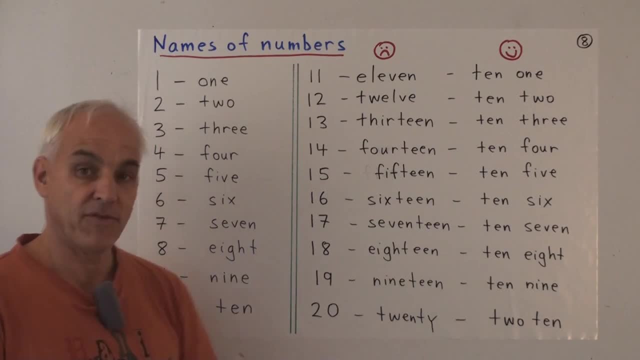 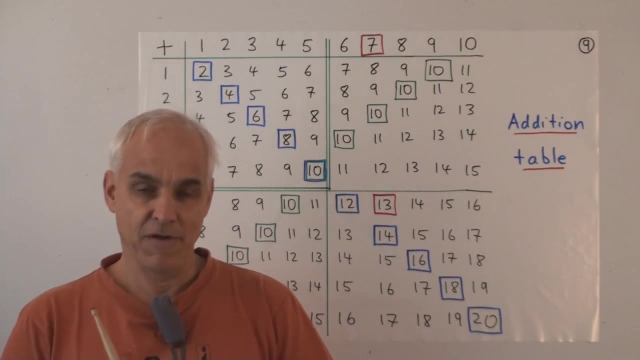 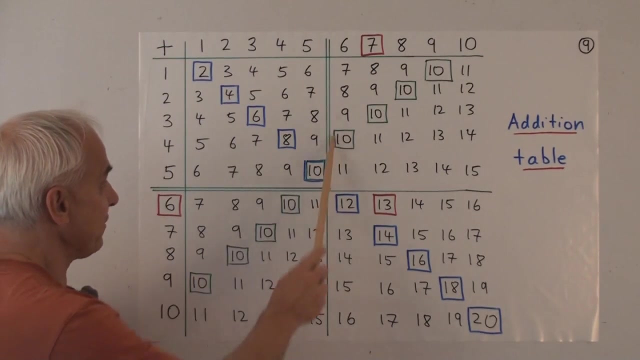 able to translate, But just to get you used to thinking about this as an alternative possibility. So here then is the full addition table for numbers in the range 1-10.. And again, it's not like our earlier addition table, which, in fact, is just here in the top. 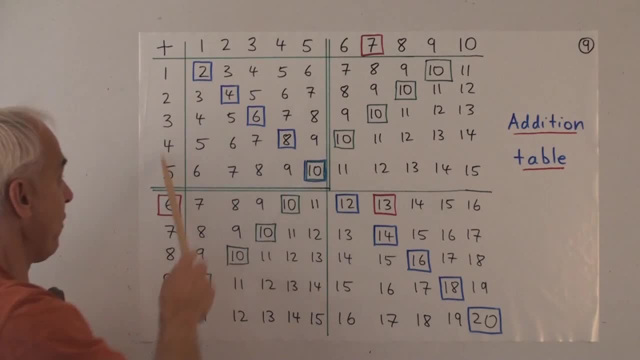 left hand corner. that's exactly a repetition of what we were talking about before, But now we're extending it so that the numbers go not from 1-5 but up to 10 in both directions. So, for example, if we want to know what is 6 plus 7, we go down here, down the first column. 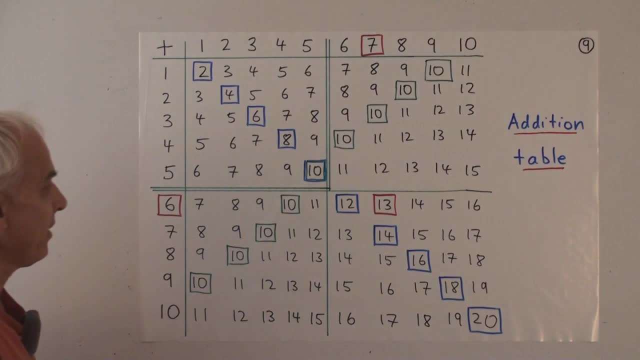 to the 6, across this first row to the 7.. And then we look in the number y we go up to in that corresponding row and column where they meet. that's 10, 3.. So 6 plus 7 is 10, 3,. 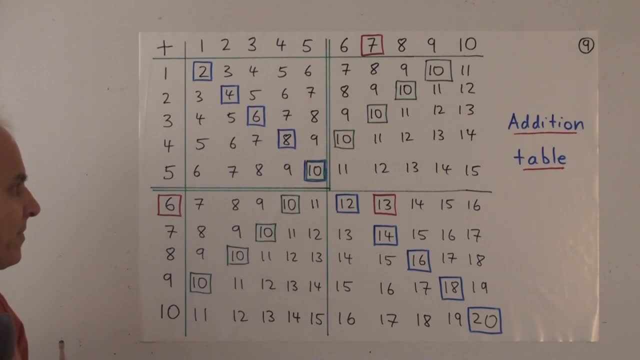 or 13 if you insist, And many of the features of the earlier table that we were talking about are replicated here in this larger table. The pattern is really the same, it's just that everything gets extended. So, along every row, we're still increasing by one. Along every column, we're still increasing. 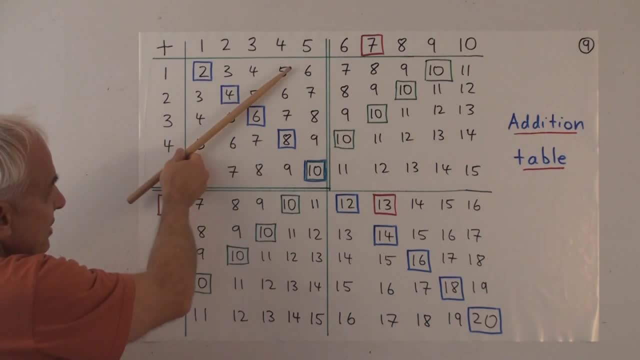 by one as we go down Along these cross diagonals. the values are still constant. And along this main diagonal we're going: 2, 4, 6, 8, 10, 12, 14, 16, 18, 20.. That's the standard. 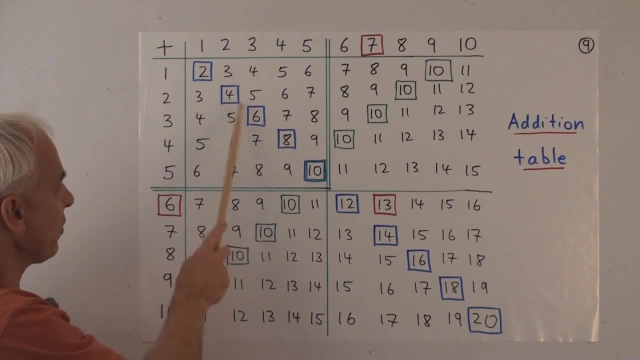 terminology- Simplified terminology: 2, 4, 6, 8, 10, 10, 2, 10, 4, 10, 6, 10, 8, 2, 10.. There's another aspect of this that I want to point out, another important. 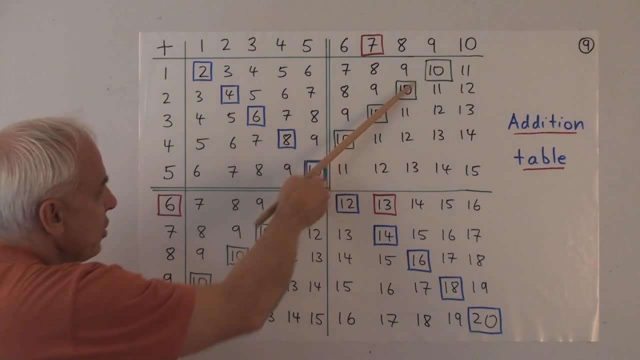 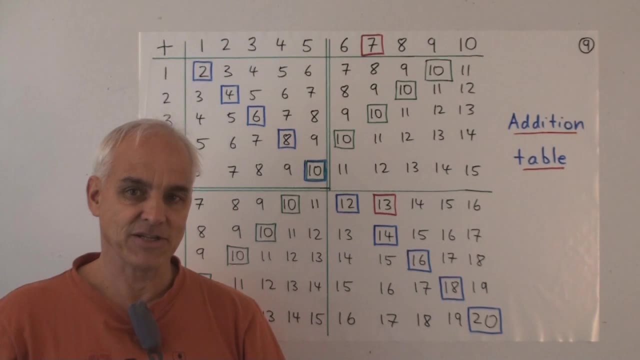 sort of cross diagonal, which is this one right here. So when students learn this table, of course takes them quite a long time to learn it. This is not something to be done in a week. This takes months to learn. This is not something to do for most young people, But this particular cross diagonal is, I think 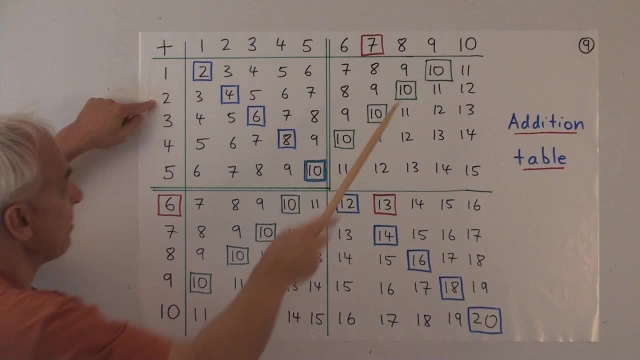 very helpful. Here are the places where the two numbers add up to 10.. So 1 plus 9 is 10, 2 plus 8,, 3 plus 7,, 4 plus 6,, 5 plus 5, and then symmetrically 6 plus 4,, 7 plus 3,, 8 plus 2, and 9 plus 1.. 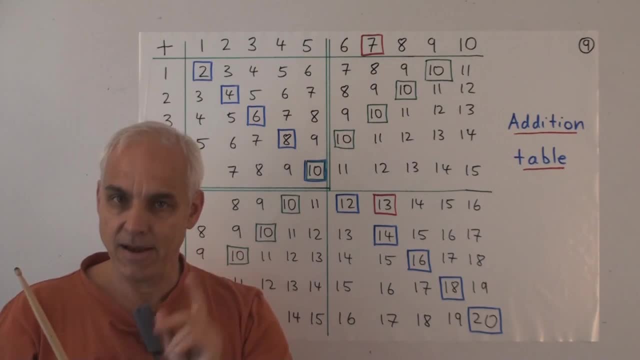 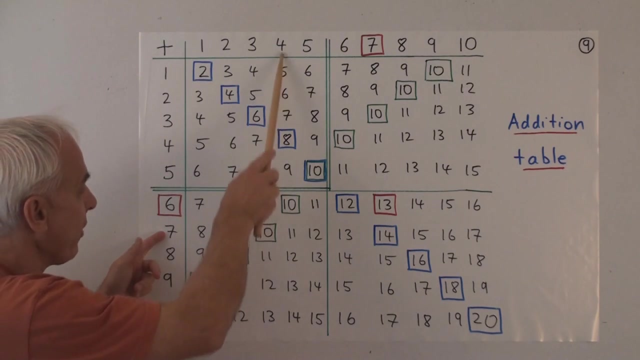 Those are the various combinations of two numbers that make 10. And those are kind of an anchor or sort of some fundamental points that I think add some structure to the table. So, for example, if you want to know what 7 plus 4 is, 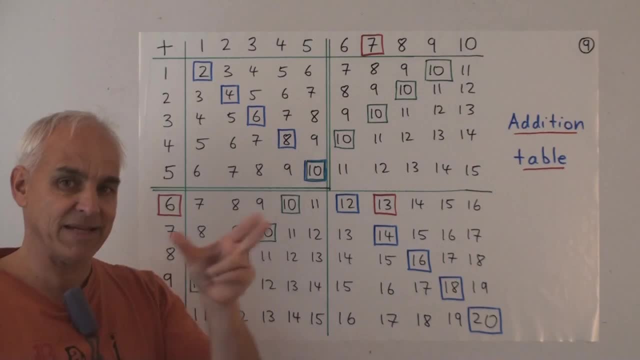 if you remember that 7 plus 3 is one of those important combinations that makes 10,, then 7 plus 4 will be 1 more, so it'll be 10: 1. While 7 plus 5 is 2 more, so it'll be 10: 2.. 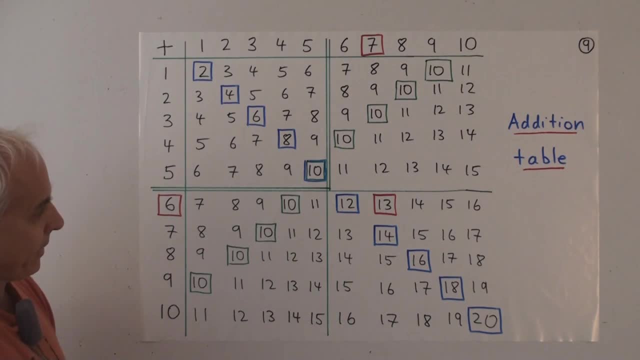 So, again, the same comments that I made about the earlier table apply to this one. I don't have any particular suggestions on how students have to learn this table, but learn it they must, And they must learn it in such a way that it becomes rote. 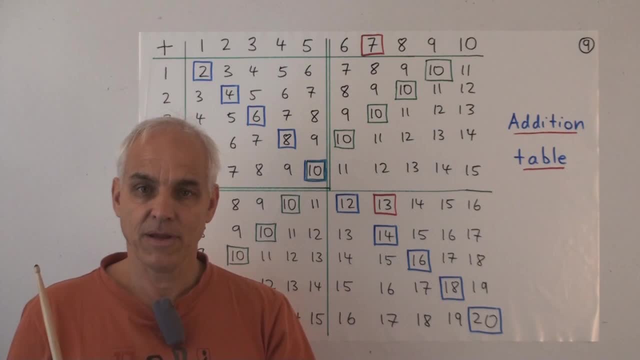 that it becomes so ingrained that they know the answer immediately, without having to pause and think. So although it's nice to have students thinking independently and making discoveries, it's also very important for young people to learn things by rote, if necessary to repeat them over and over again until they learn them. 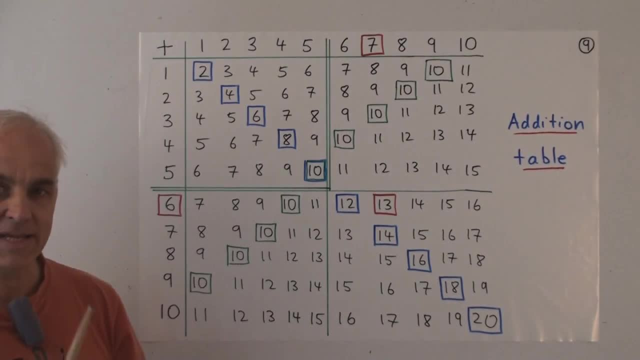 At first. they should be aware of the reasons for any entry. They should know, or at least be able to compute and check for themselves, that if you take 4 and 8,, for example, then you do really get 12.. Or 10, too.